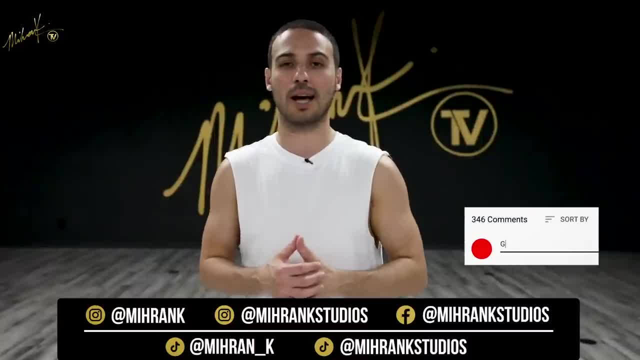 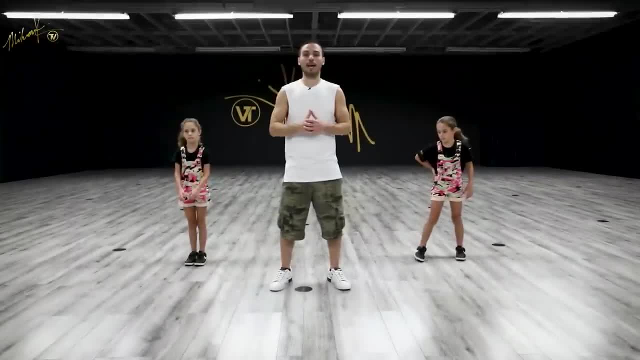 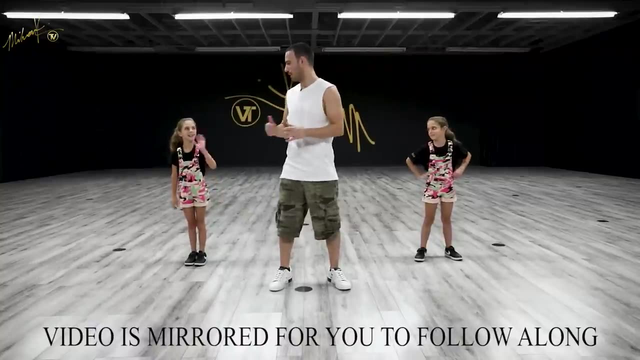 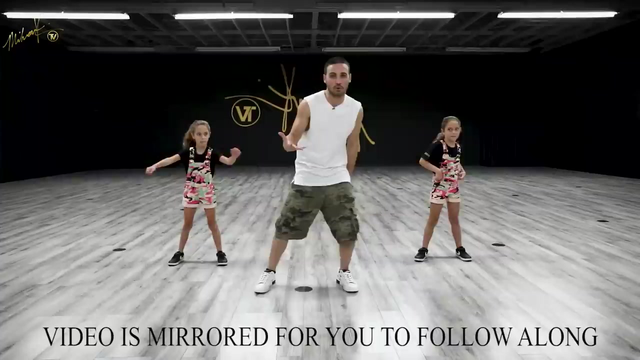 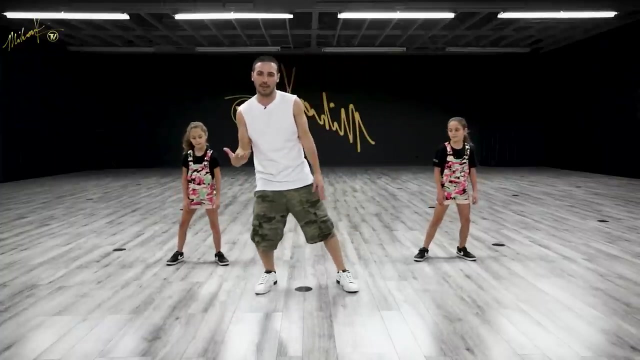 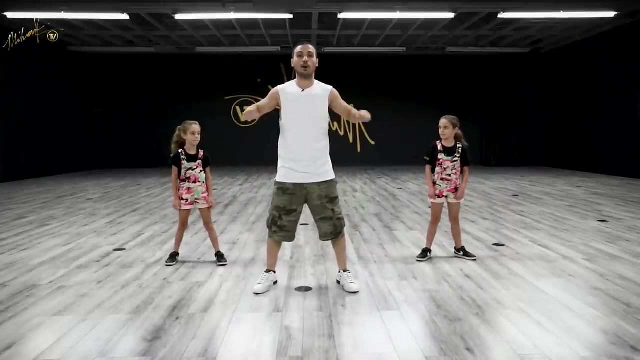 every single time we release a new video. Also, leave your comments in the comment box. Let us know what you thought of this video and what else you would like to see on this channel. Let's get started. Arms, we're going to go out, they're going to go cross, and then we're going to bring them up. 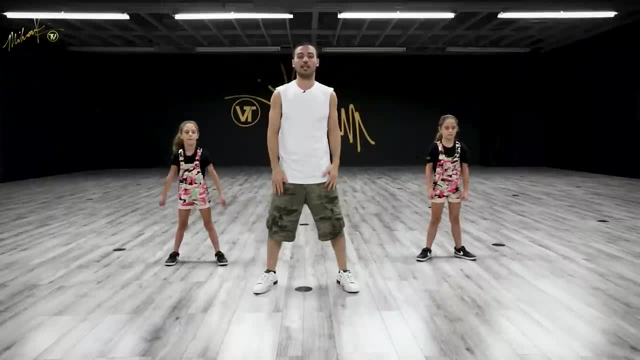 out and cross Again. six, just the arms. Six, seven, eight. Let's go out, cross out, cross. Awesome, Let's do that again. Five, six, seven, eight. Go out, cross out, cross, Perfect Now. 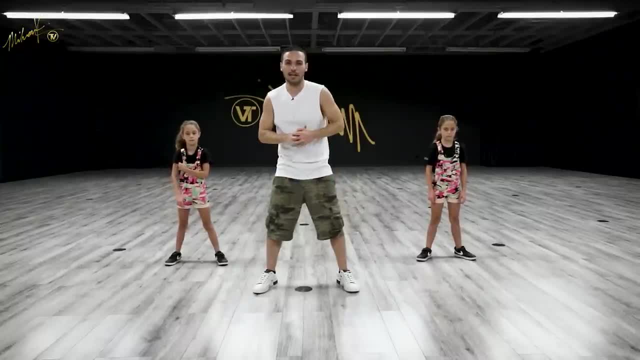 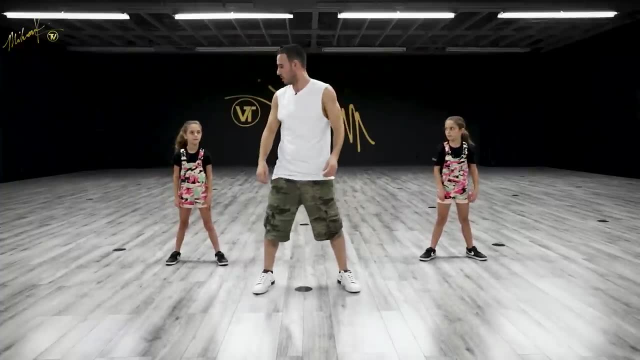 let's put the arms and the feet together. Here we go. Six, seven, eight. We're going out and cross and out and cross. Perfect, Let's do that a couple of times Together. You ready, girls? Here we go. Five, six, seven, eight. Let's go Two, three, four. 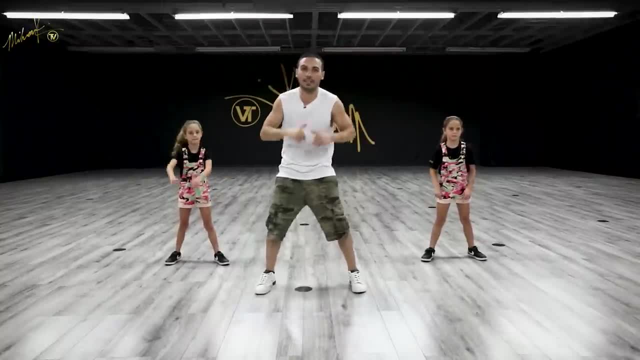 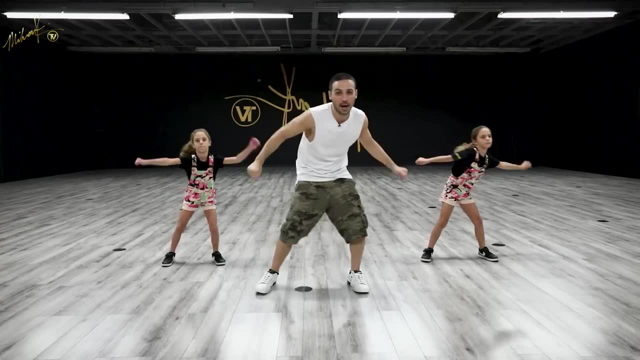 Perfect Again. Five, six, seven, eight, Go one, two, three, four, Good One last time. Five, six, seven, eight, Go out, cross out, cross, Perfect. From here I'll show you the feet first. 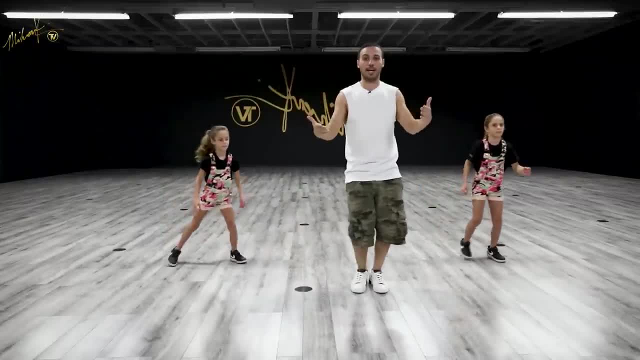 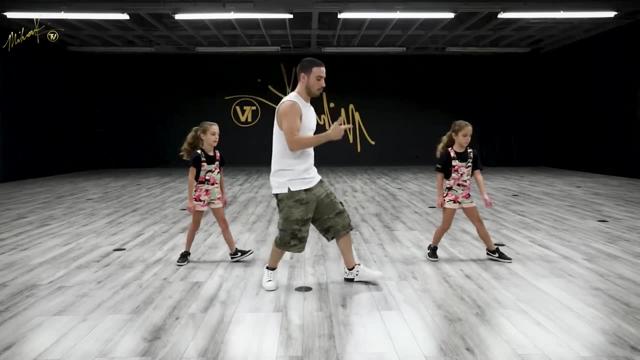 You ready, ladies? We're going to go step and together, and step and together. Good, That's great. Let's do that again. Six, seven, eight, Go right, left, left, right. Good, As I'm stepping. 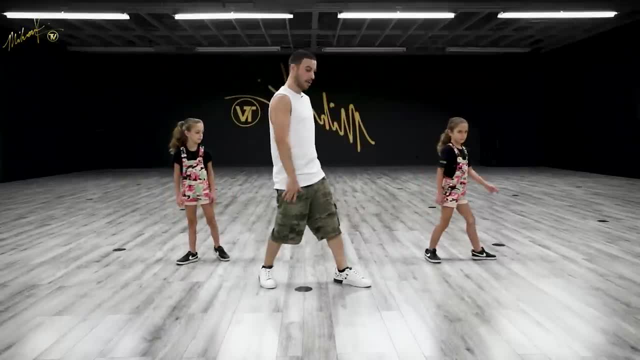 to the side. I'm turning my body a little bit. Let's turn Whoop. Then we're going to turn back to the front. Then we're going to go whoop, turn back to the front, Perfect, I'm just showing you. 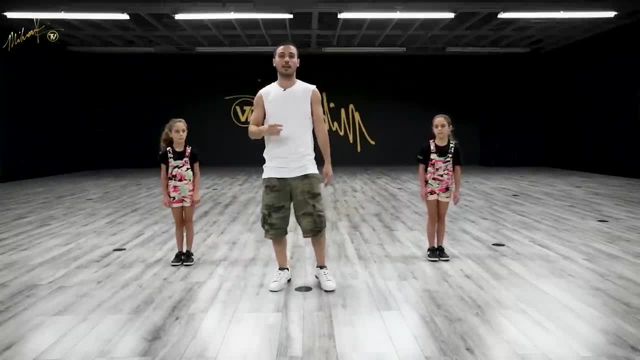 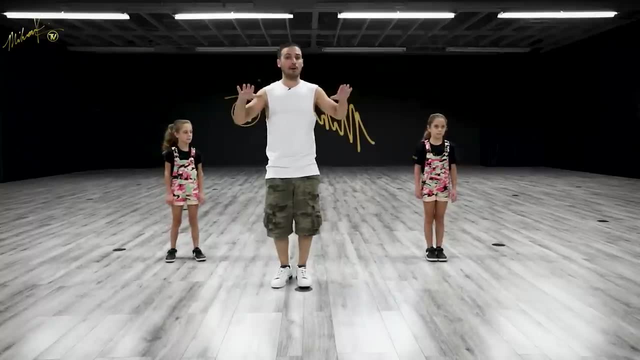 the feet now, and then I'll put the arms together One more time for the legs. Six, seven, eight, Go, step, step, step, step. The one thing I want you to make sure to do is keep that bounce, because if 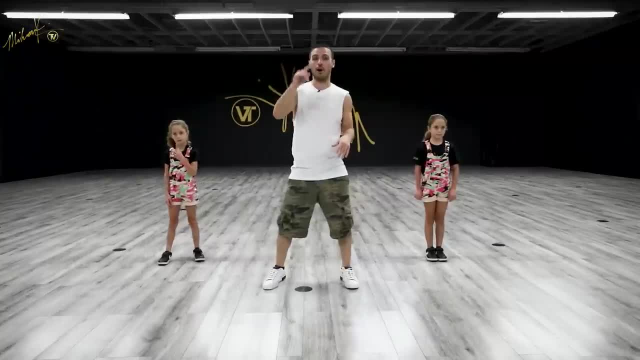 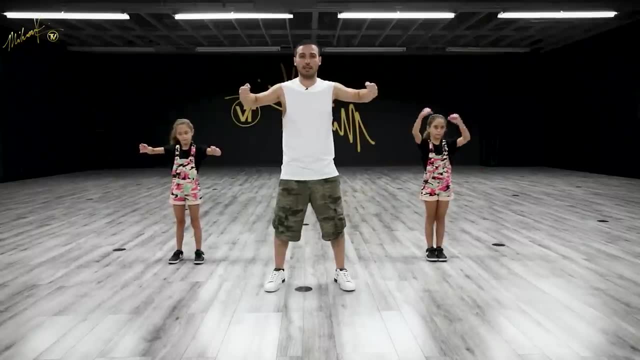 you came from the bounce, then we want to keep that bounce. If you came from the bounce, then we want to stay there, as we're going side to side. Your arms, arms only. We're going to shoot across the body and then we're going to go boom straight down, keeping the elbows up, just like this. Then 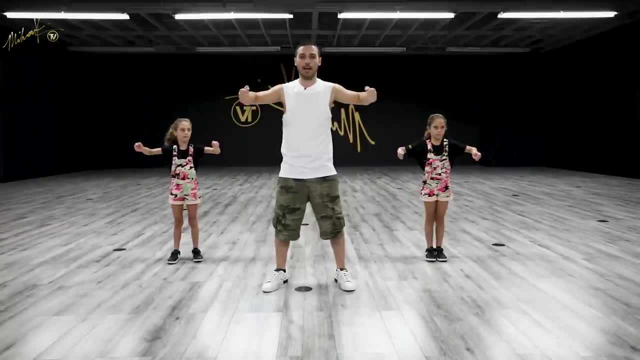 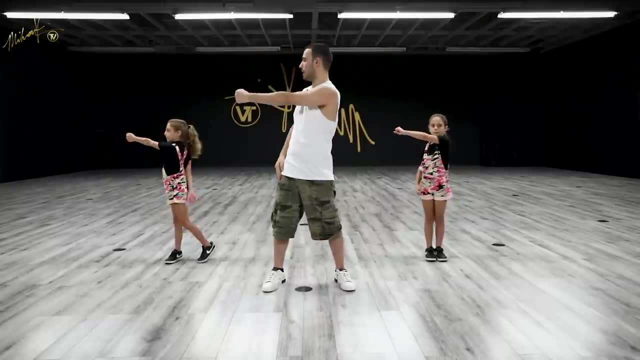 we're going to go out to that side and then boom arms back down. One more time for the arms, Six, seven, eight. Across the body and down. Across the body and down. Awesome Now when you throw. 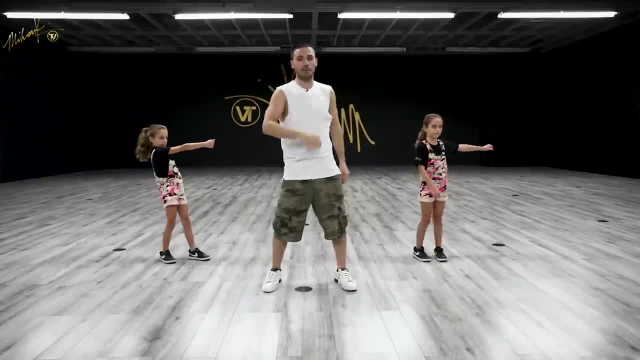 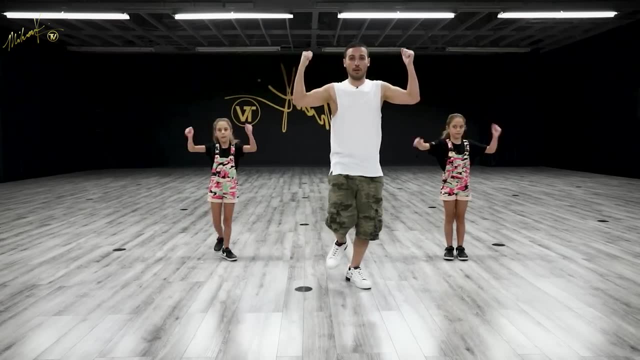 the arm, lean away from it just a little bit. I'm going to throw the left arm and I'm going to lean away from it. I'm going to step, and then I'm going to step together, Boom, and then I'm going to go. 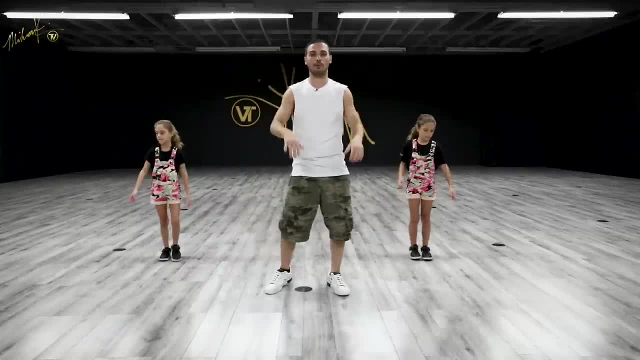 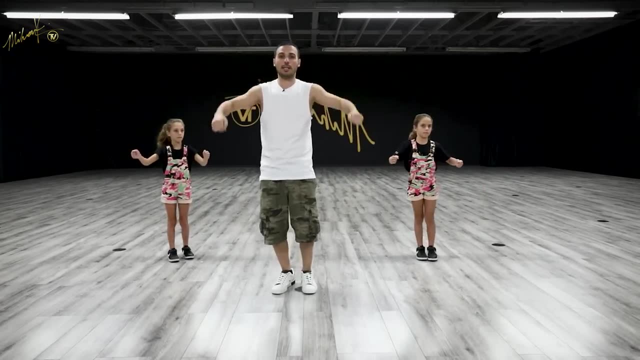 whoop. step together, Boom, Go ahead. Let's do the legs and the arms together. Six, seven, eight. We're going. one and two, three and four, Again, five, six. Keep that bounce. Go, boom, boom, boom, boom. 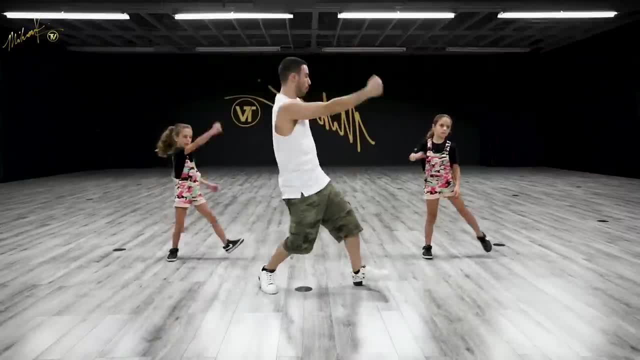 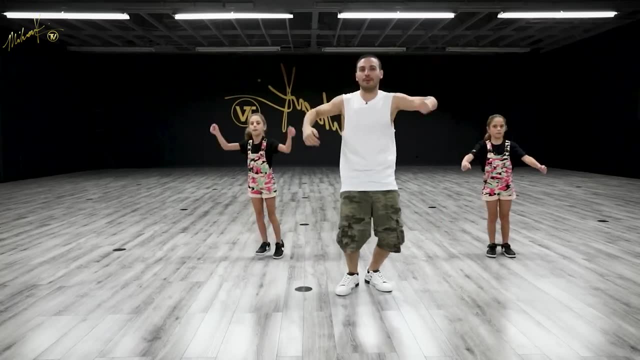 Again five, six, seven, eight. Go one, two, three, four, Again five, six, seven, eight. Keep the bounce, bounce, bounce, bounce. Let's do a recap of everything so far, from the very top Six, let's: 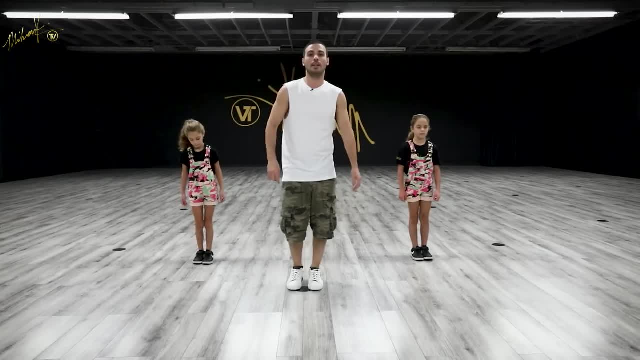 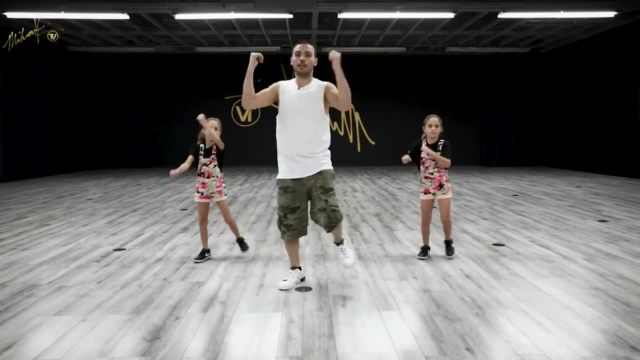 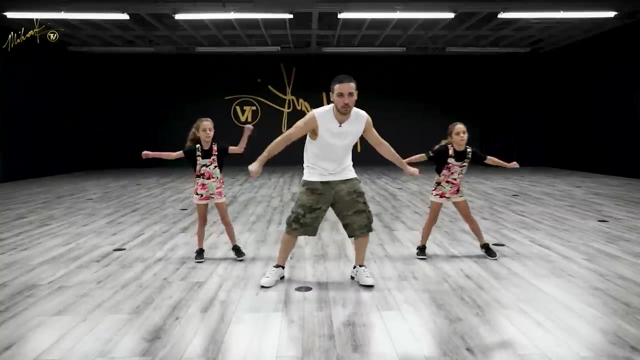 go feet together. We'll step out into the move. Six, seven, eight, Step one and a. two, three and a four. Step five, six, seven, eight, Perfect, Let's do that two times together: one, five, six from the bounce: Go whoop, whoop, whoop, whoop, Go. step two, go, step four Again. 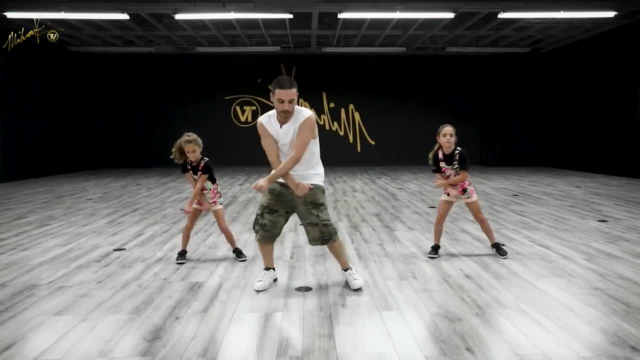 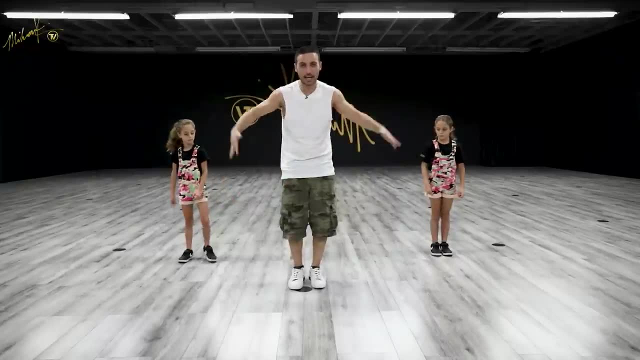 five, six from the top, Go bounce. two, three, four, Go five, six, seven, eight Awesome guys Moving on from here, Feet together, Arms are up. We finished right here. Ladies, you ready, We're. 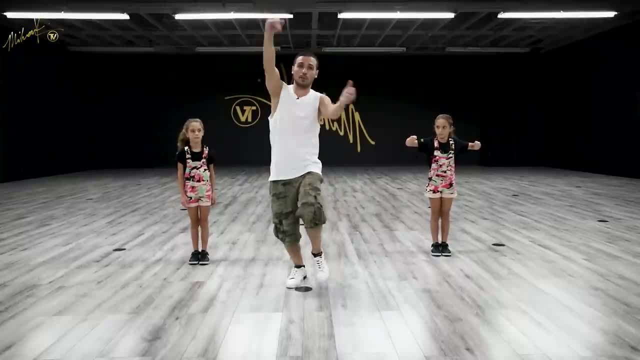 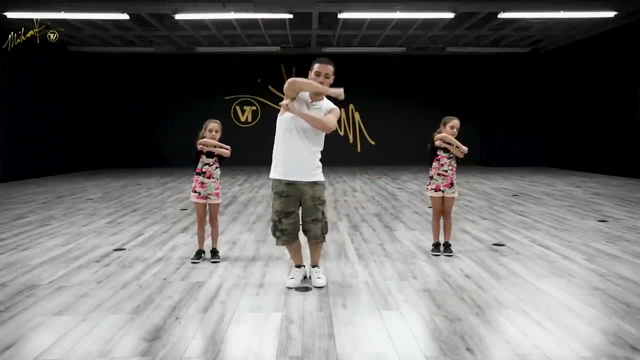 going to step out with the right leg. We're going to bring up the left arm. We're going to go one, Yeah, fix your body And then slide it in two. You're going to stay on the side. Left arm is going to be on top. 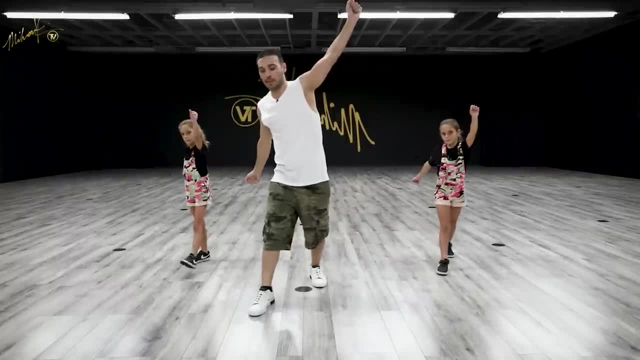 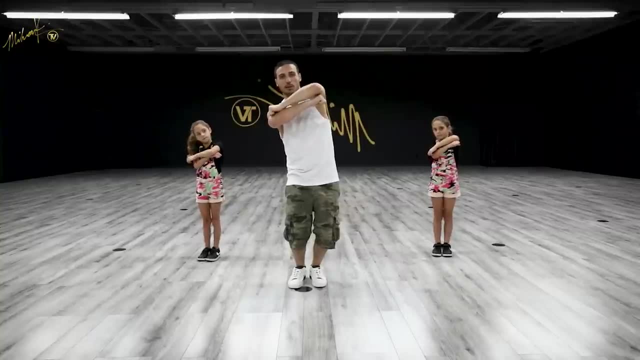 right. Perfect. Now we're going to switch the side. Boom, Stepping out with the left leg, Lily, left leg, Yep. And then we're going to slide it back and boom, Stay on that side. Now the right arm is on top. Let's do that. move a couple of times, okay, Six, seven, slow. This is one. 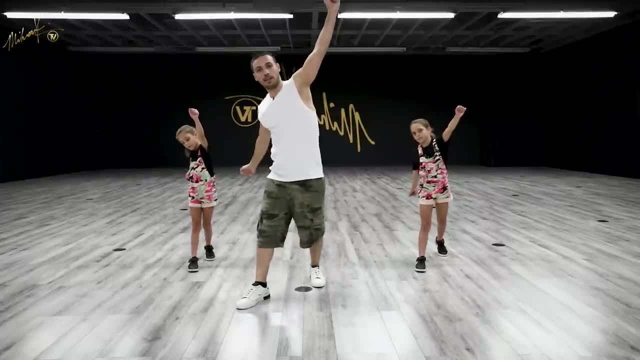 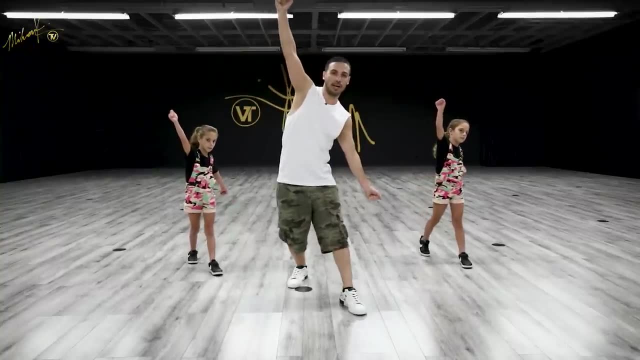 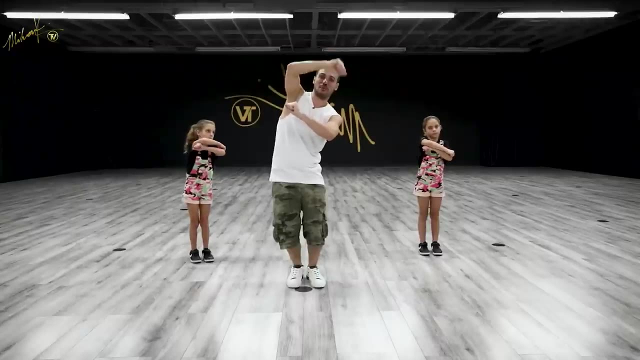 This is two, This is three, This is four, Perfect Again. five, six, seven, eight. And hold, Good, Let's make sure we got the correct arm up, Sophia. good, Lily, good, Let's slide it back. Whoop, Hold that, Make sure that same left arm that was up is on top now. 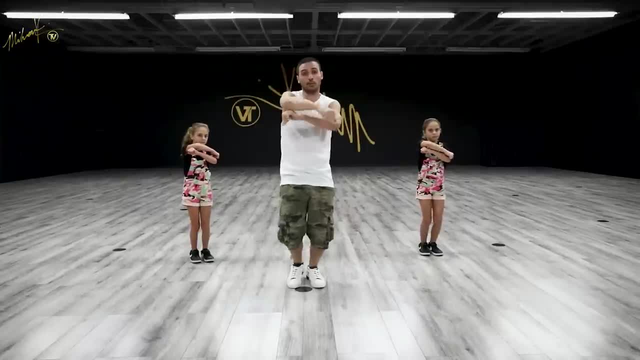 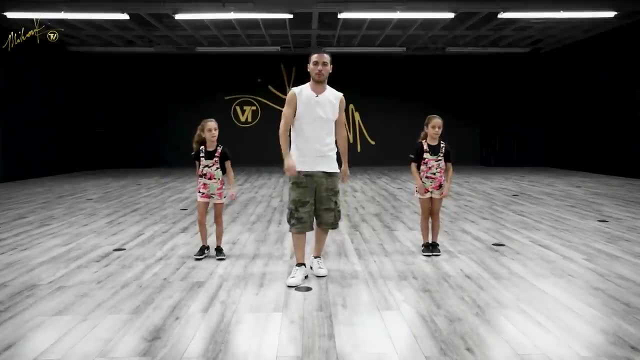 right, Good job, bend your knees, ladies. We came from the bounce to the other side. Whoop, Good, Perfect, Slide it in, Boom, Awesome. Let's do that a couple more times. a little bit more tempo now, Just that move. six, seven, eight. Step one and two, three. 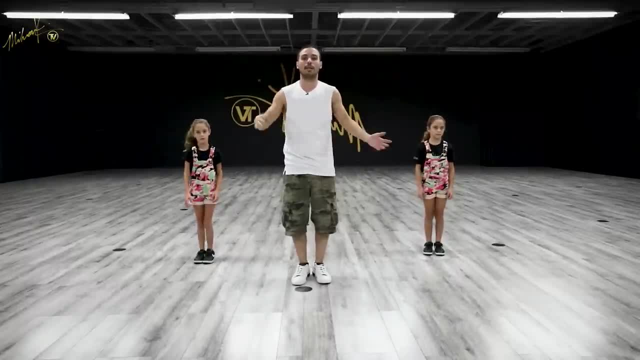 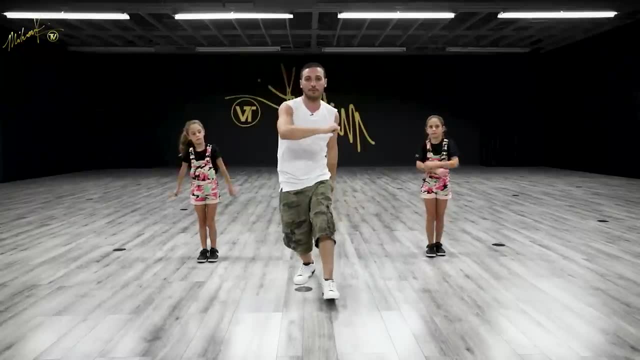 and four. good again. six, seven, eight and one and two, three and four. perfect. from here we're going to do four quick steps, five step, six and seven and eight. good, let's. 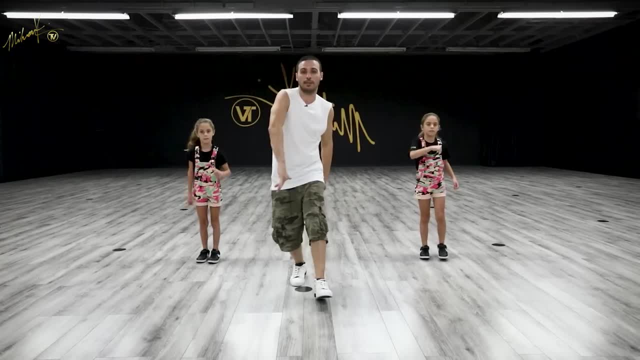 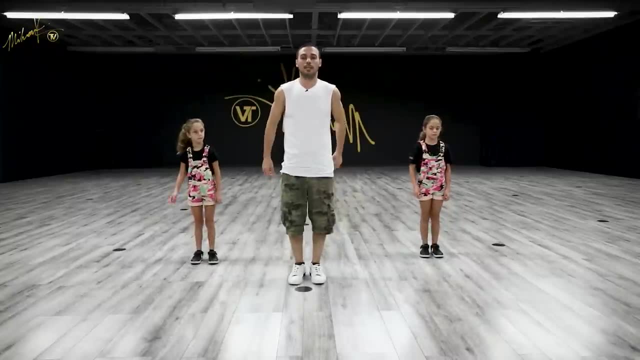 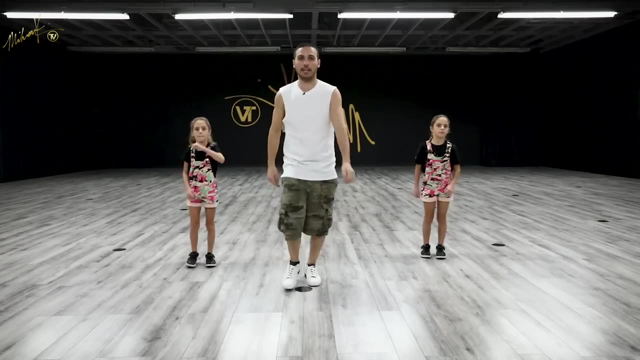 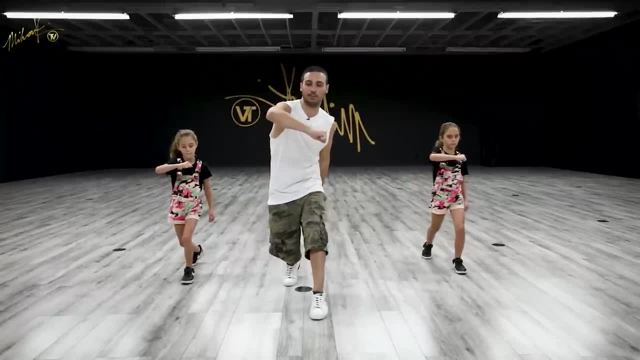 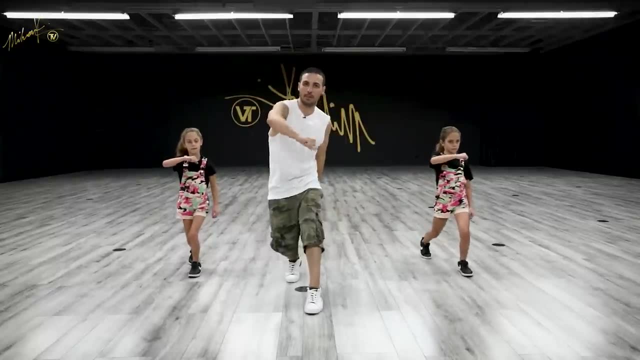 with the right leg, left arm comes up: whoop, let's all hold that. make sure we all have that. bring it back, switch, whoop, bring it back, switch, step, bring it back and step, bring it back. good, but these are fast, so you're going to go slow. and then 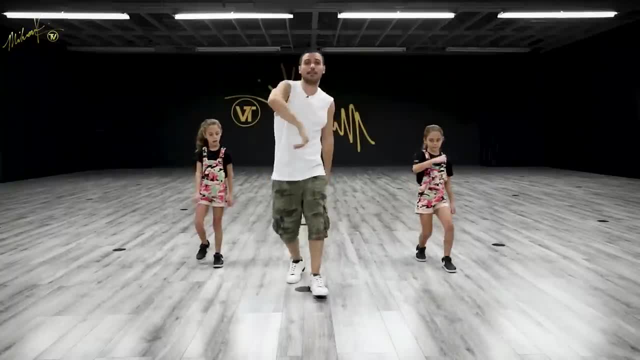 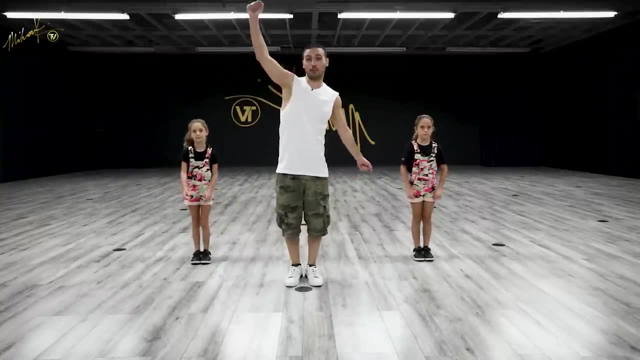 slow, and then fast and fast, and fast and fast. good, let's do that a couple of times. girls, you ready, ready? so here we go. five, six. we're going to go from the slow, slow. 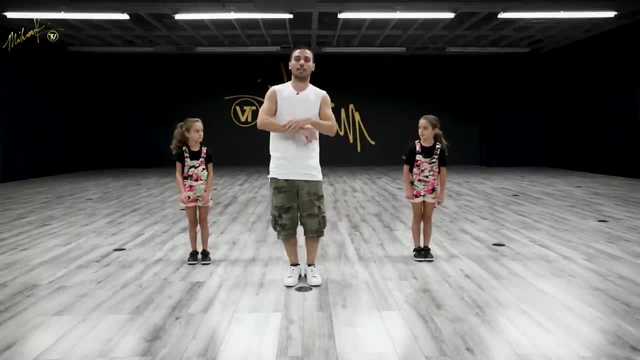 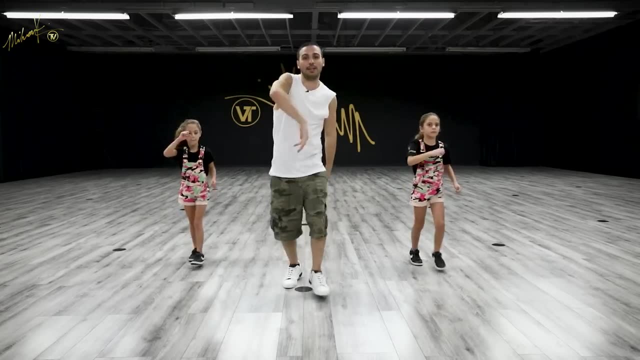 fast, fast, fast fast. five, six, seven, eight. this is one and two, three and four, five and six and seven. and hold good, let's do that again. five, six, seven, eight. 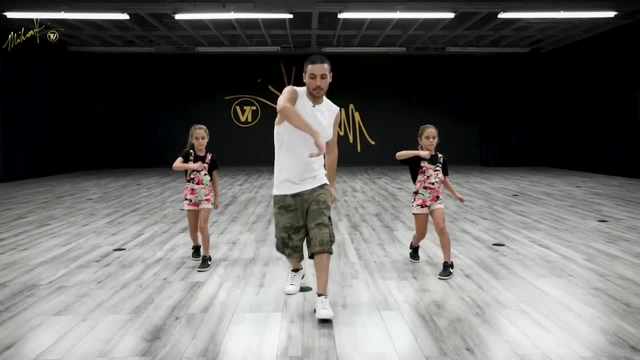 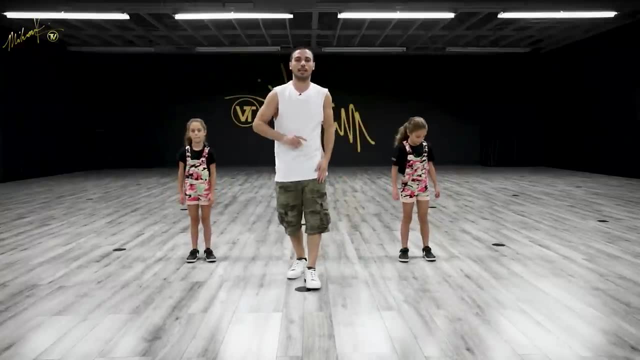 and boom, Boom, two, boom, four. step and step and step and hold good one last time for everybody. here we go: five, six, seven, eight go one, two, three, four, five and six and seven. 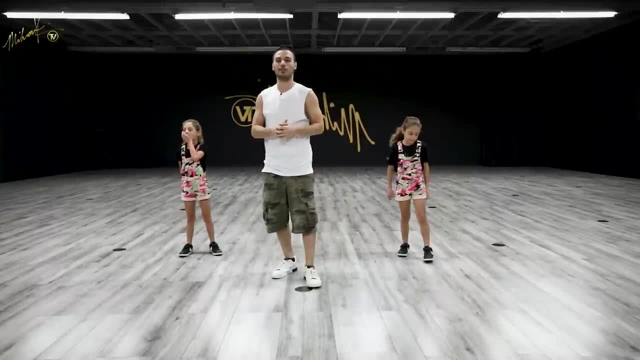 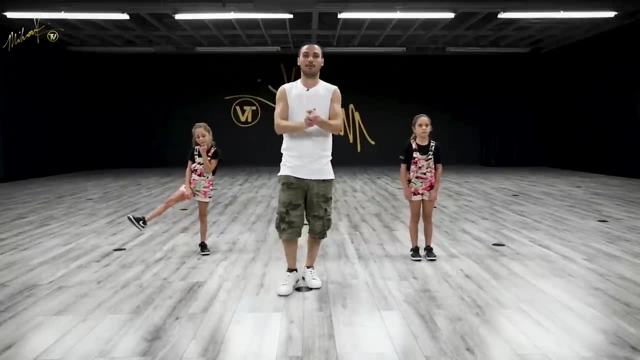 and hold awesome guys. we're already halfway there, so let's take it back to the very top, walk it slow, walk it tempo, try it with music and then move on. okay, here we go. five, six slow from the top girl. 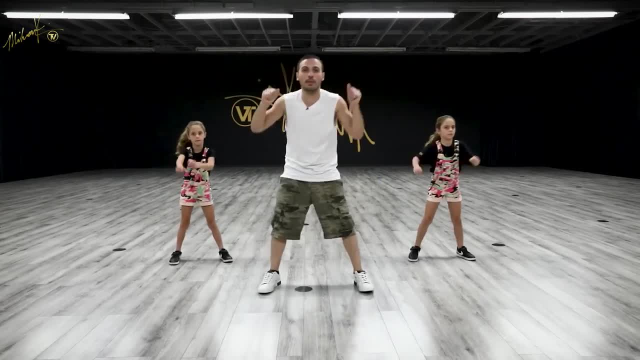 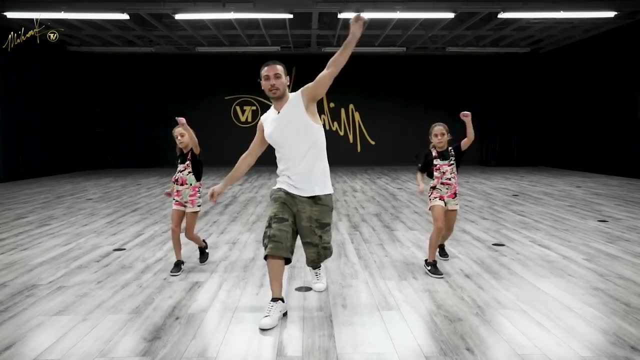 six, seven, eight. we're going bounce two, three, four, five, six, seven, eight, one and two, three and four, five and six and seven and hold good, let's do that one more. 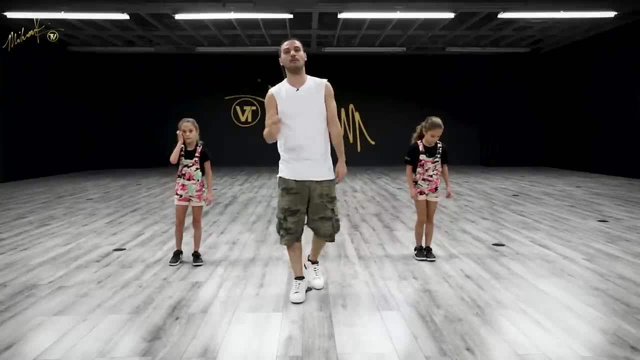 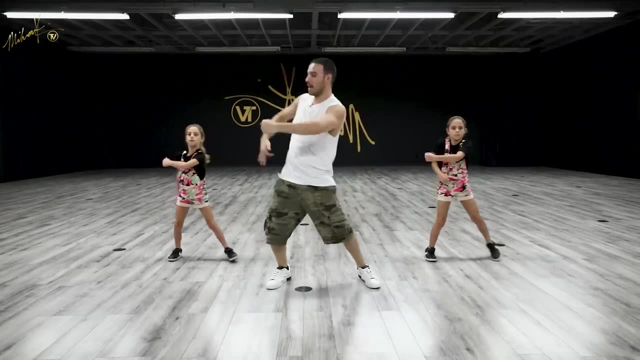 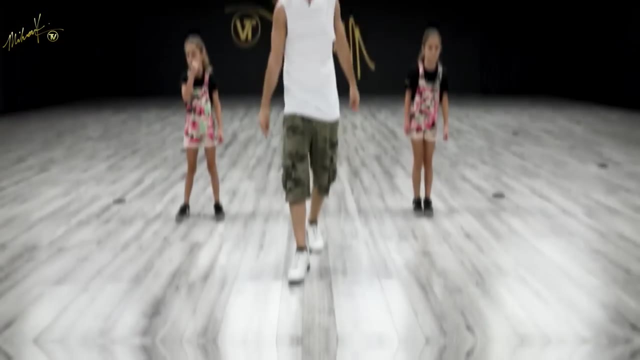 time like that now tempo, getting ourselves ready for music. five, six from the top, go bounce two, three, four. go five, six, seven, eight, go step and step and go go go hold five and six. go five, six, seven, eight, go bounce two, three, four. 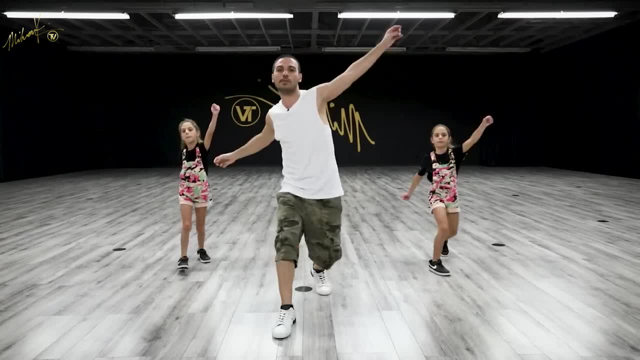 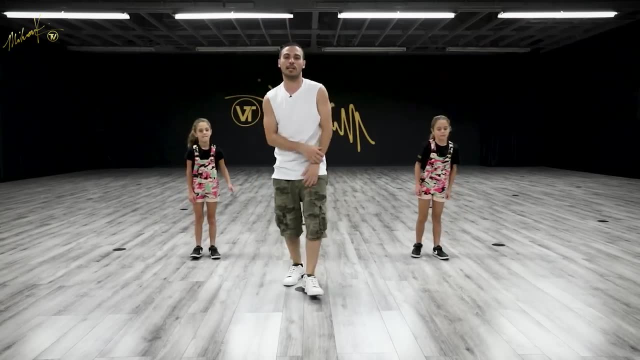 five, six, seven, eight go. one, go, two, go, step, step, step hold. good one last time, here we go. five, six, seven, eight, go, bounce, bounce and hit, hit, hit, hit, go step. 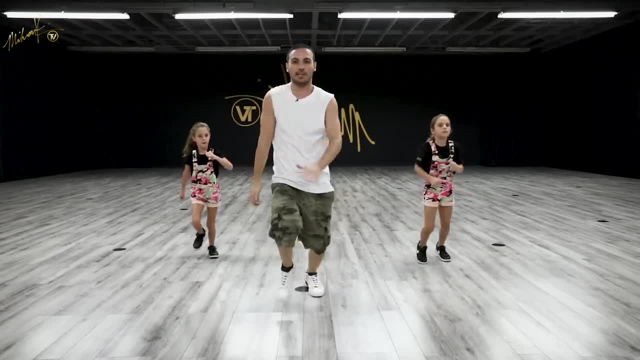 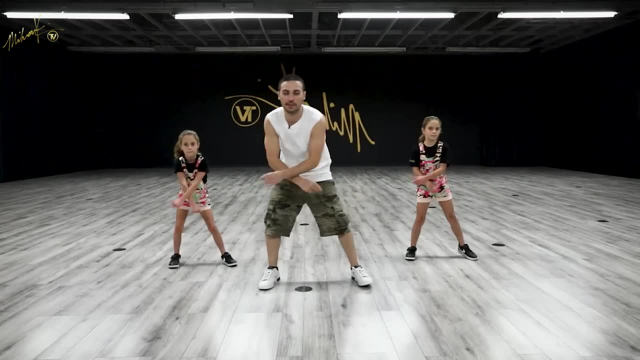 and step and go, Go, go, go stop. quick review from the very top and move on. girls from the top six, seven, eight. we're going one, two, three, four, five, six, seven, eight. step one: 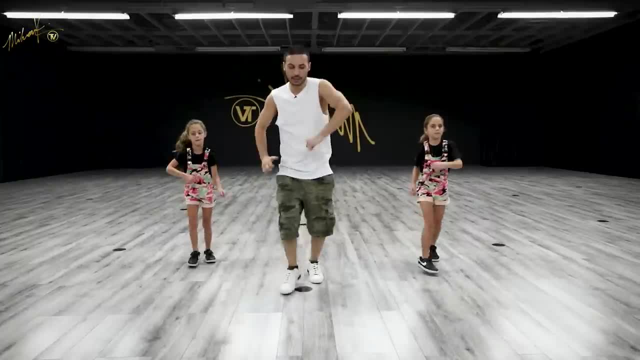 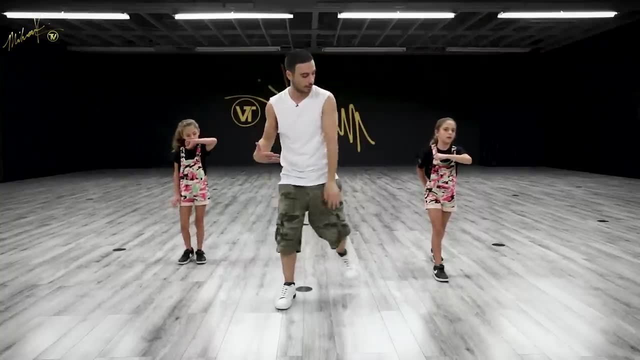 two, three, four, five, six, seven. stop, good, from here we're moving on to the right side. we're gonna swing the right arm. well, I'll show you the legs first. we're gonna go step. 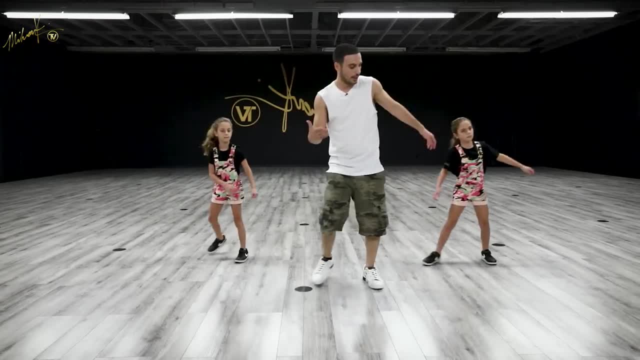 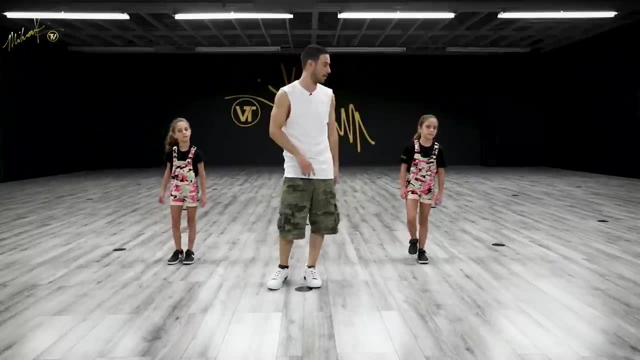 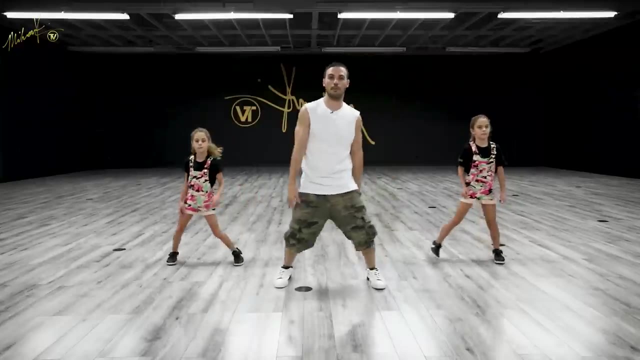 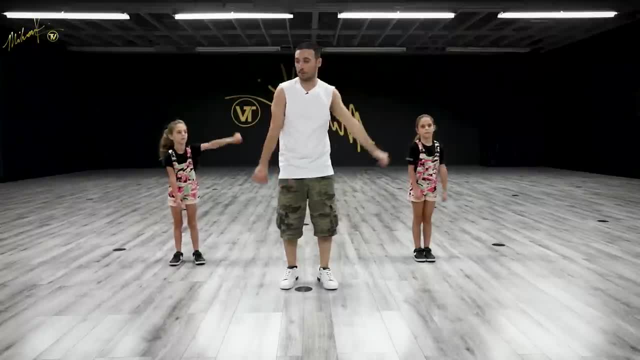 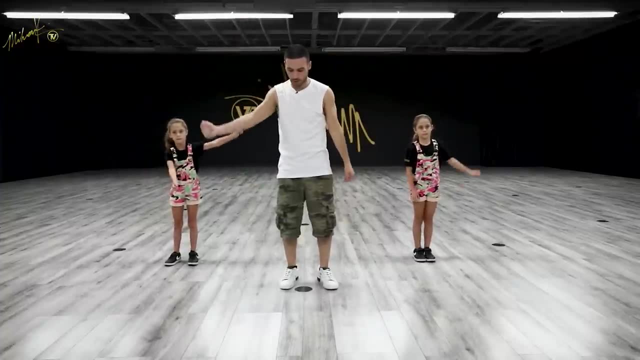 You're gonna swing and pull down, swing and pull, swing and pull, swing and pull. Good, You want to kind of make it look like once the one arm is coming down, the other arm is coming up. Okay, So, starting with the right arm, Six, seven, eight, Go. 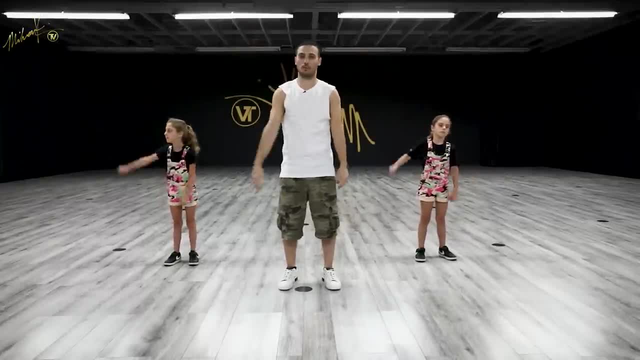 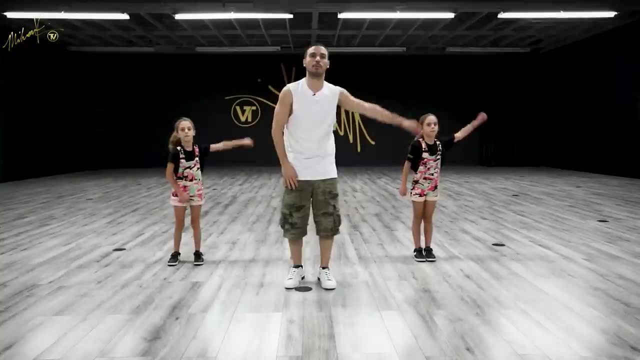 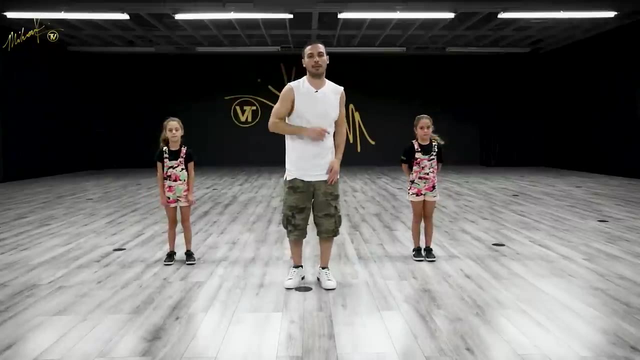 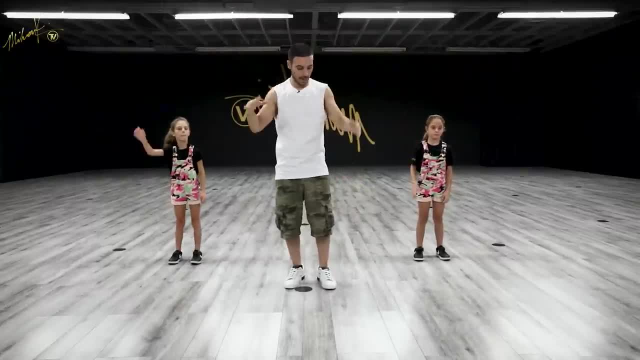 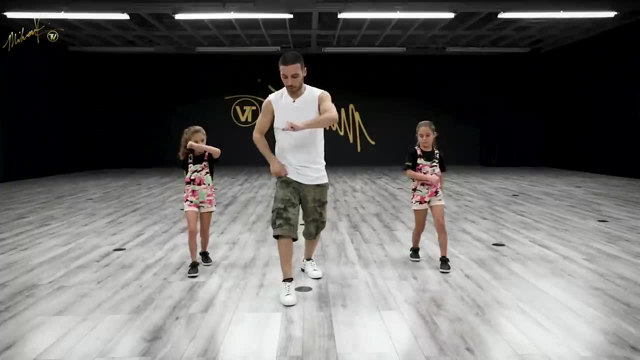 snare, boom, six, seven, eight. Good, Now the arms in the middle Legs together, going side to side. Remember we went five, six, seven, eight. So we're left leg in front, right Switch the leg, Sophia, Right arm up. We're gonna go to. 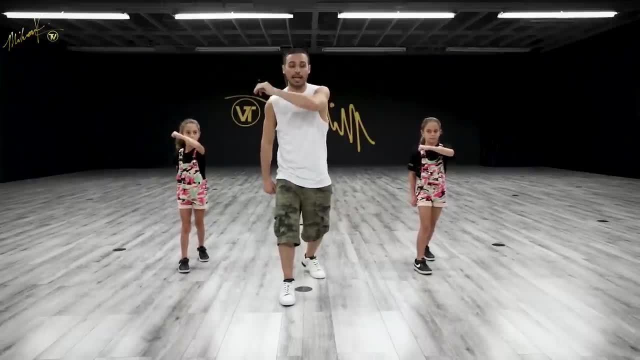 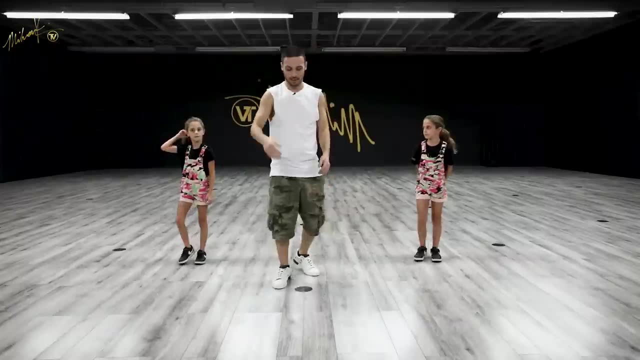 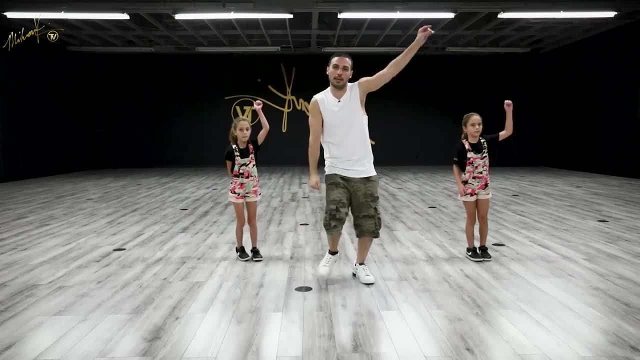 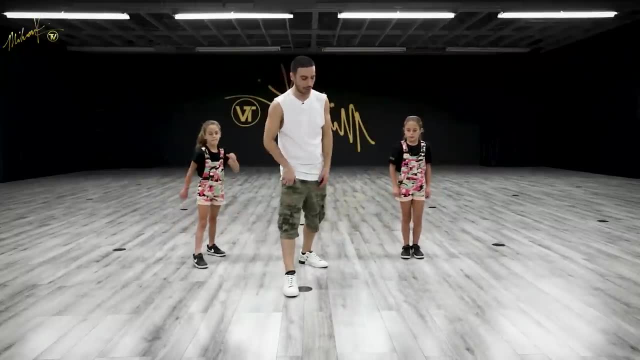 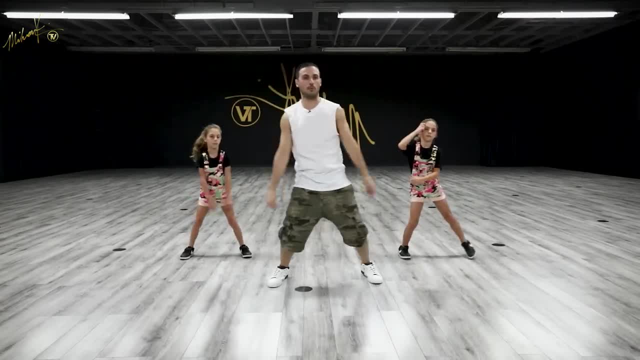 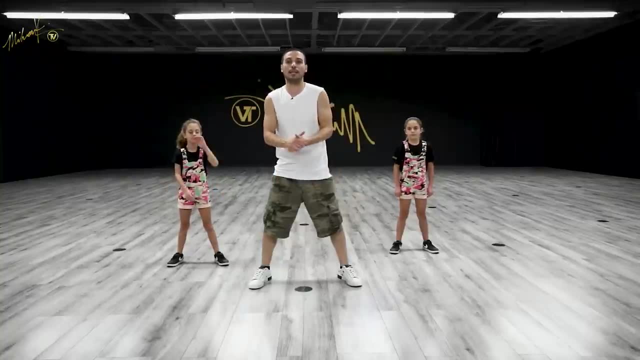 eight, Go Boom. two, boom, three, boom, six and a seven, eight Awesome guys. Let's take it back to the very top Five, six, seven, eight, Go bounce. Two, three, four, Go boom. 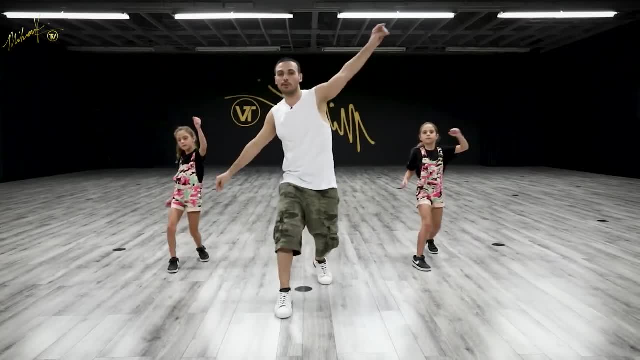 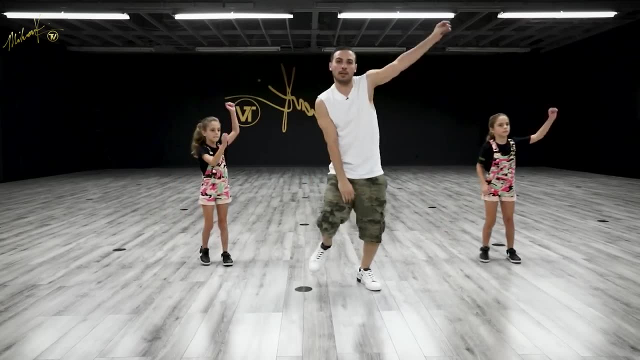 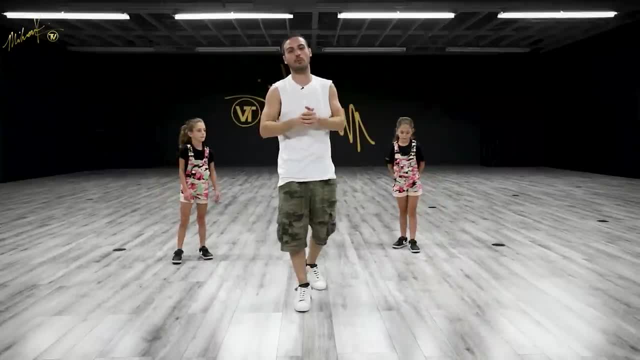 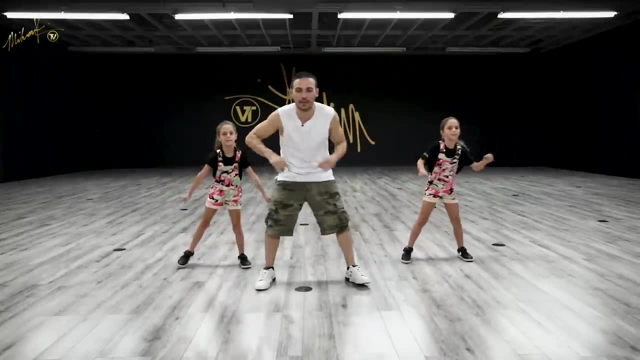 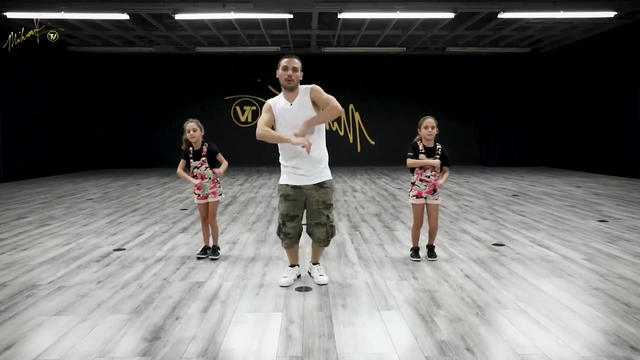 pull. Good, Let's do that two more times, Get really comfortable with it and finish the routine up. okay, Here we go, ladies again, Five, six, seven, eight Go bounce Two, three, four, five, six, seven, eight Go. one, two, three, four, five, six, seven. 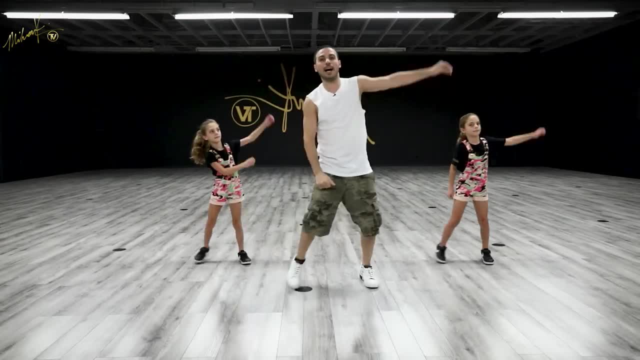 eight. Go one, two, three, four, five, six, seven, eight. Go one, two, three, four, five, six, seven, eight. Stop Good, One more time, just like that, and we will finish it. 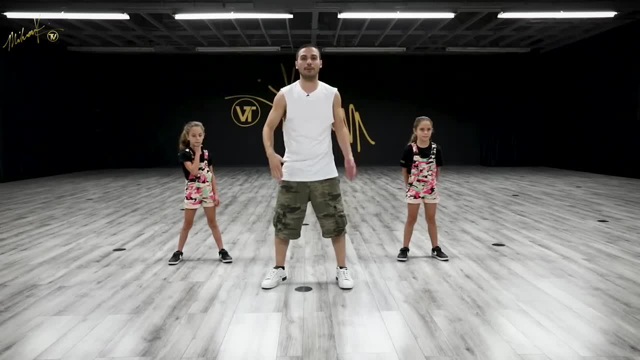 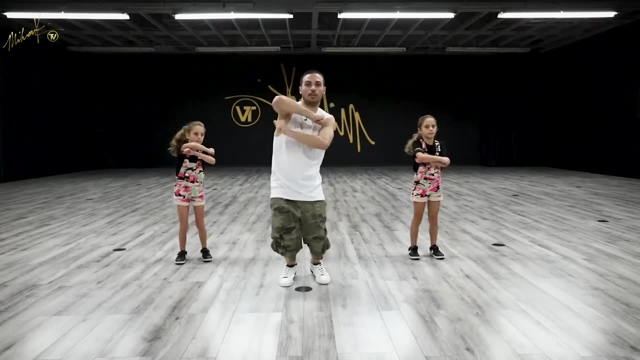 up to the last eight count. Here we go: Five, six, seven, eight. Go one, two, three, four, five, six, seven, eight, Go one, two, three, four, step and step and step and step. 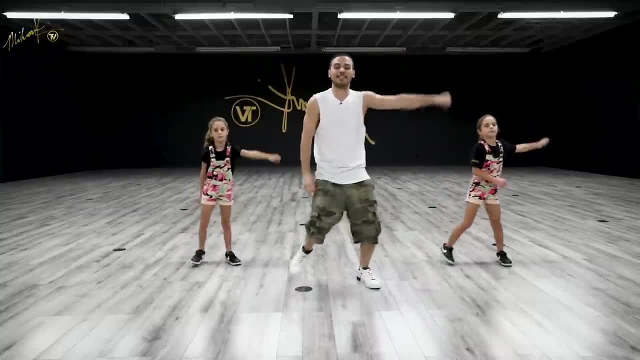 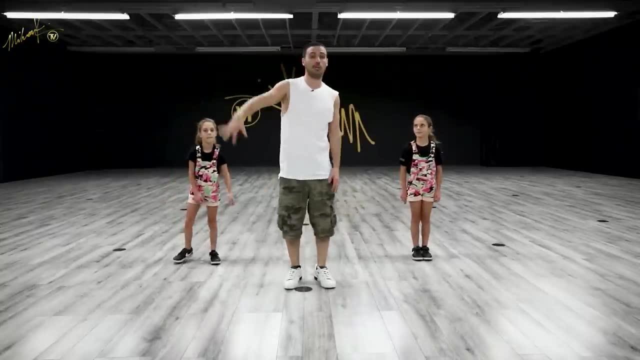 Go one, two, three, four, five, six, seven, eight. Good job, guys. Let's move on from. I'm going to show you guys the arms first. Okay, you guys ready? ladies, Here we go. We're pulling on one. 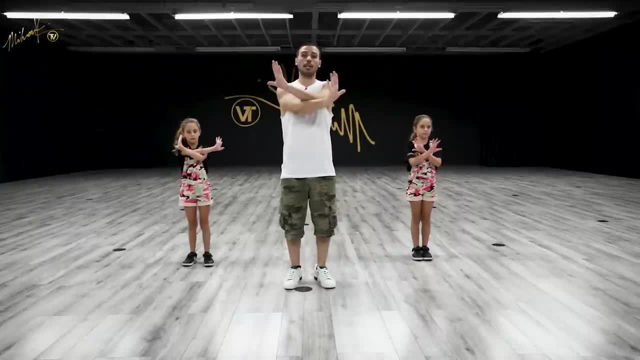 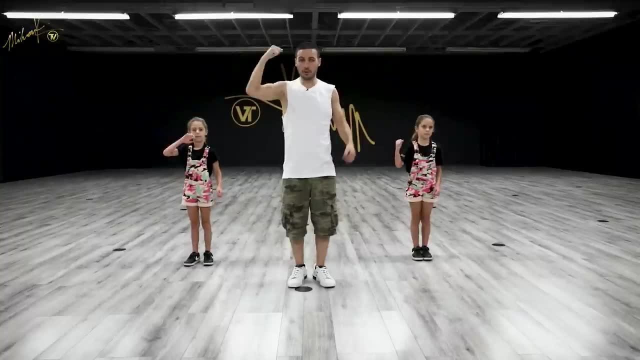 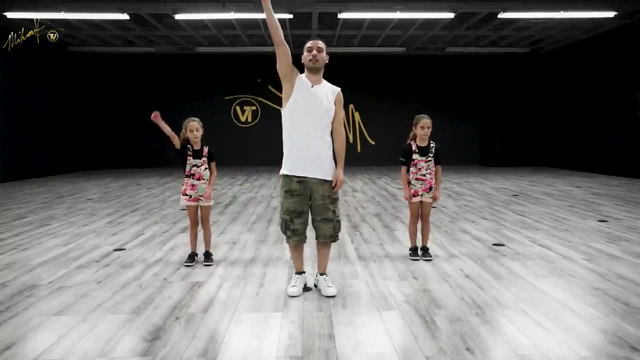 We're punching on two, We're crossing on three. Open on four. Good Again, five, six, just the arms. Go pull punch cross open Five, six, seven, eight, Go pull punch, cross open Five. 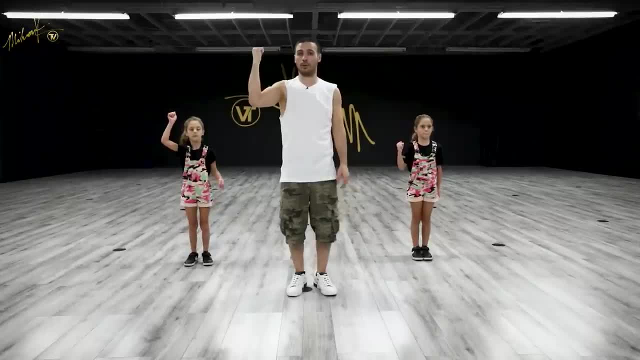 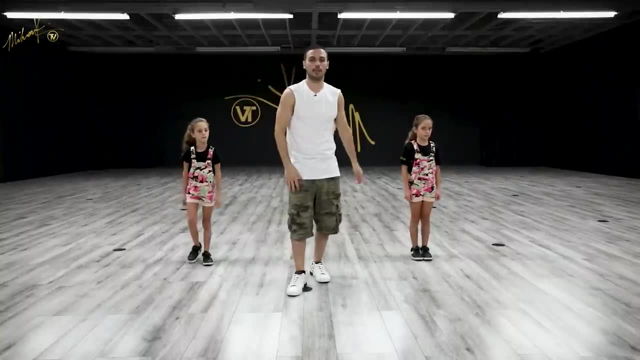 six, seven, Slow. You're going to go pull, You're going to go punch on the cross. Your hands are going to be open. And then back to fist. Five, six, seven, eight. Go pull, punch cross. 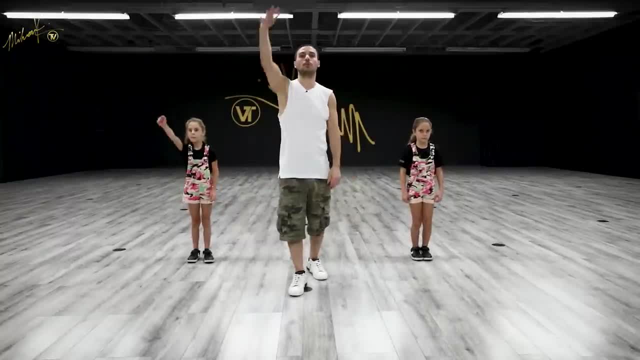 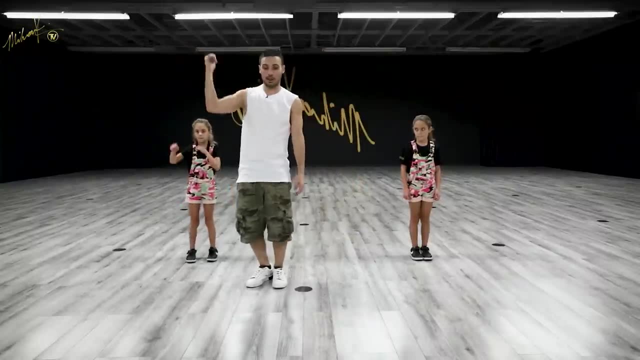 open Last time. Six, seven, eight, Go, pull, punch, cross open, Perfect Your feet. So remember we finished here. I'm only going to show you the feet, But you're going to go from here stepping. 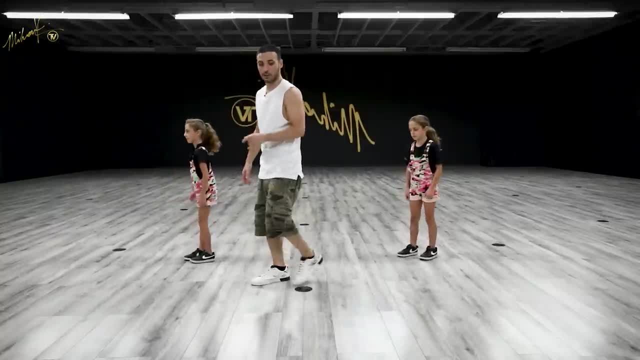 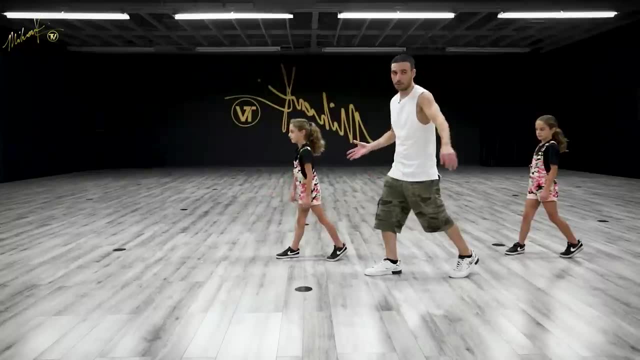 with the right leg. Your body's going to turn a little bit. Ladies, let's start. We're going to go: step right leg, step left leg, step right. The right is on the tippy toes, Left is flat And we're going to turn our. 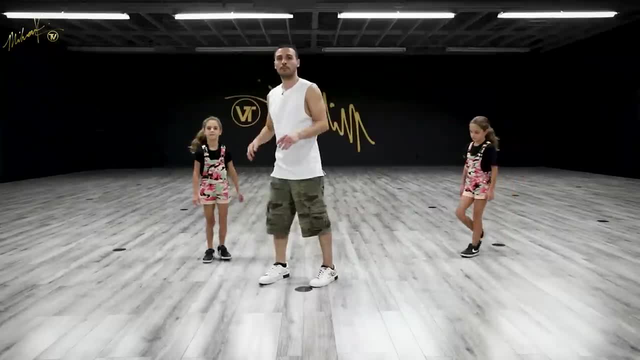 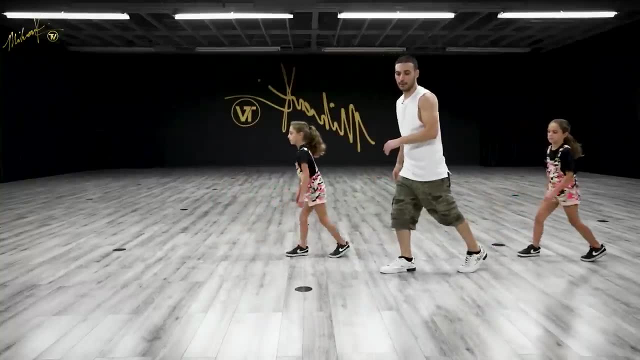 bodies around. Okay, Let's go back to our beginning position. Six, seven, eight: Step right leg, Step left leg, Step right leg And turn Good Again. Five, Let's do it sharp ladies. Six: 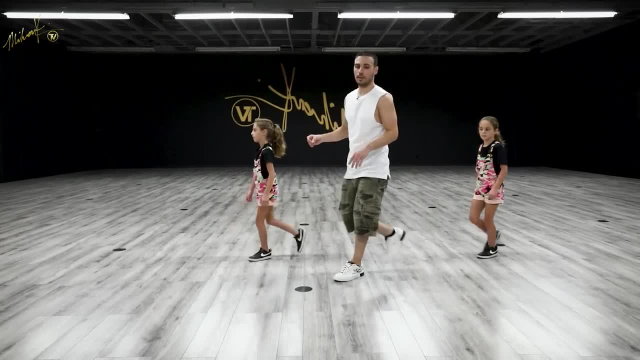 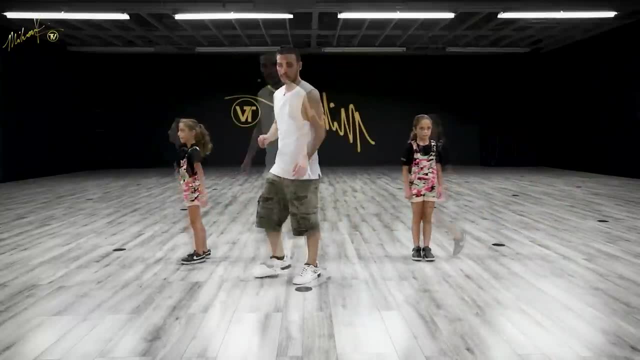 seven, eight. We're going right, We're going left. We're going right, We're going turn. Good Again, Five: Now put a little bounce to your step. Six, seven, eight. Go right, left, right, turn. 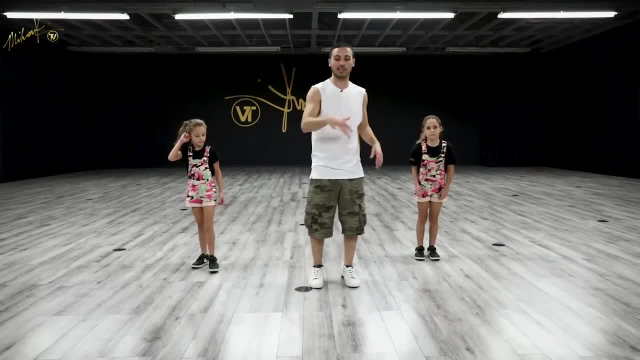 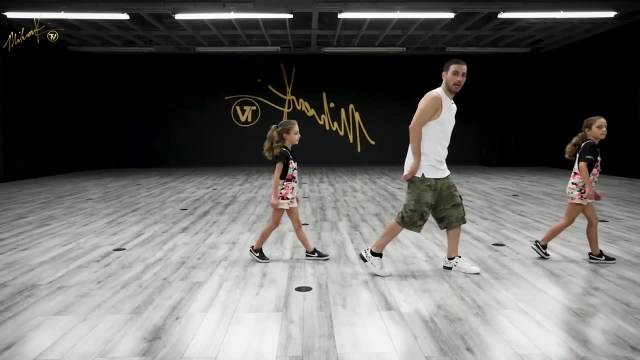 Good One last time. Here we go. So remember, the feet are together. Your last move was seven and eight. We're going to go right, left, right turn. Good, Bring it back. Here we go. Now we're going to connect the arms and the. 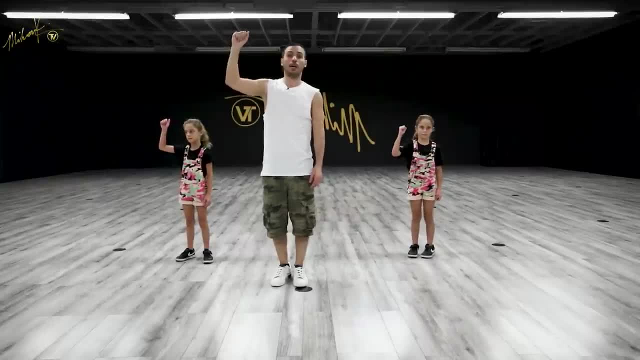 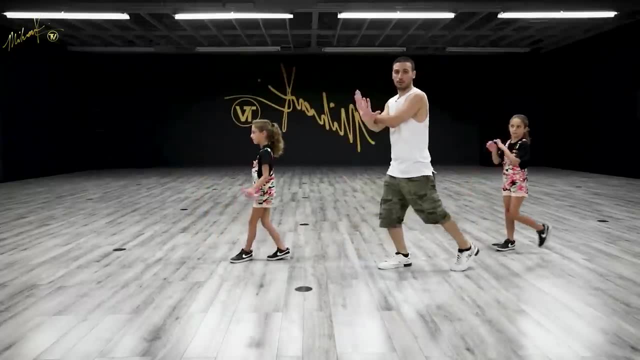 legs together. Our arms just finished on eight. Everyone's arms are up. We're going to pull back on one at the same time. We're going to go one, We're going to punch. two, We're going to cross. three, We're going to open. 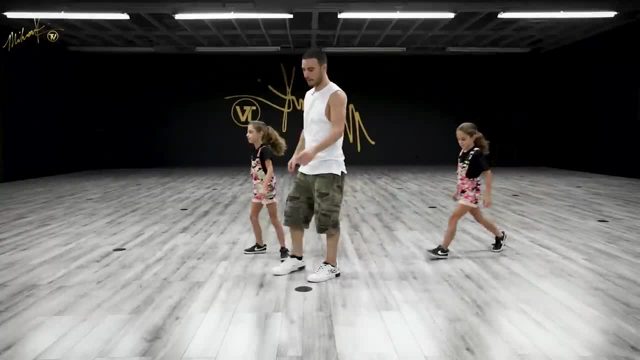 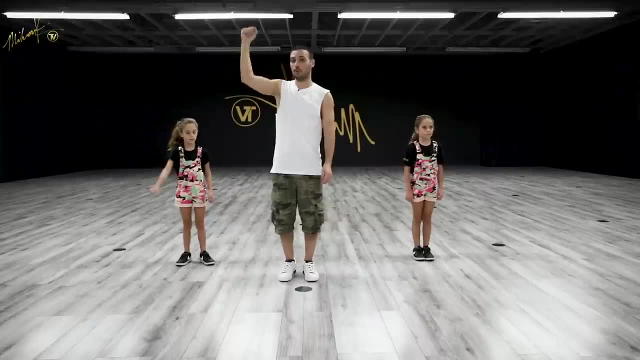 four. Good, And that's how it works. Let's try again. Five, six, four. Every time. now we're going to go five and six, seven and eight to start one. So remember, you're pulling the left arm twice. 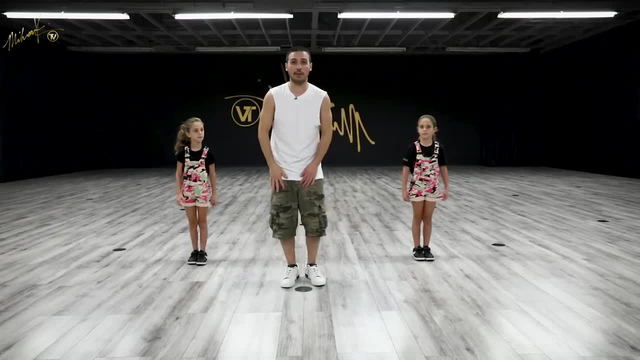 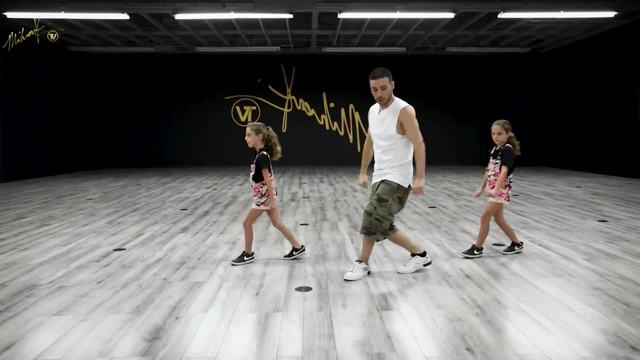 On eight and then on one. So on five ladies, Six, seven, eight. This is five and six, seven and eight. Go one, Go two, Go three, Open four. Good Again, Here we go, Same spot. 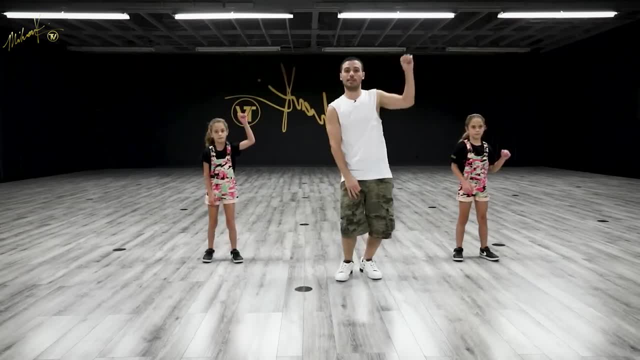 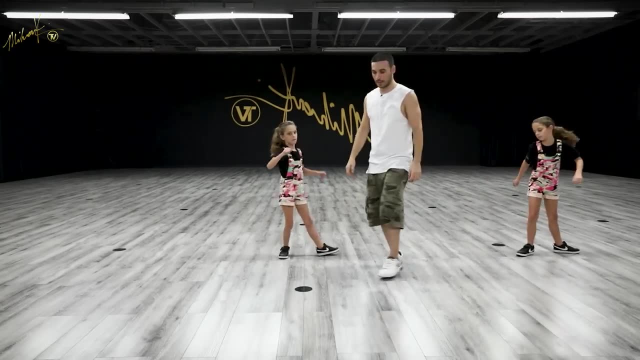 on five, Three, four, Go five and a six, seven and an eight: Go one, two, three, four. Good Connecting that really well, Let's do that a couple more times, Two more times together: Five, six, seven, eight. 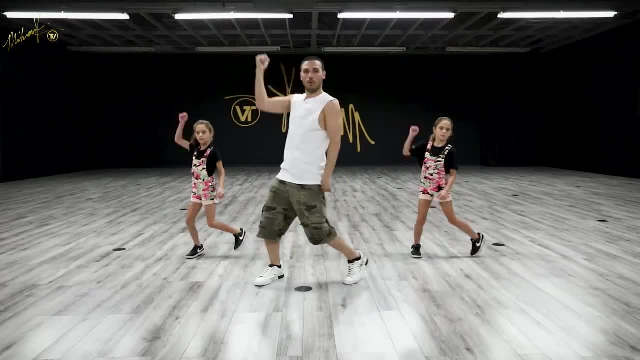 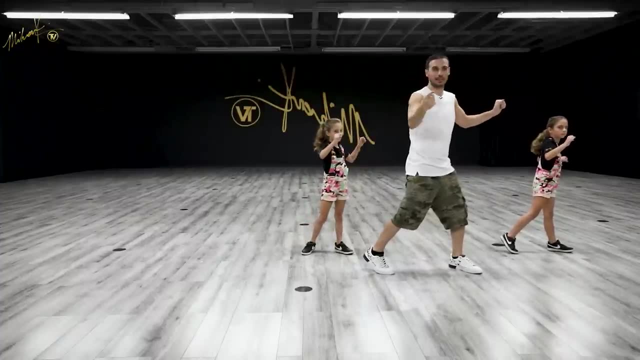 Go swing. and six, seven and eight. Go. one, two, three, four Good. Again. try to keep your focus to the front. Arms are here. Turn your body a little bit this way, Lily Good. From here, let's show them the legs. 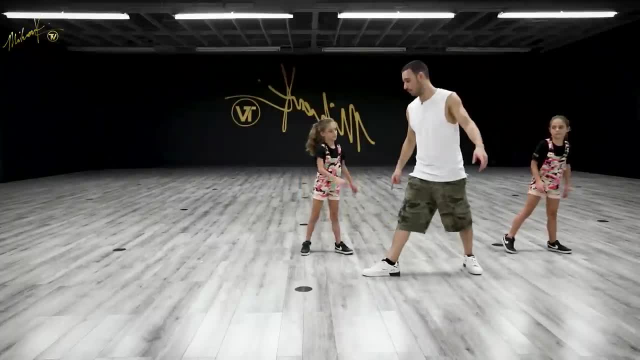 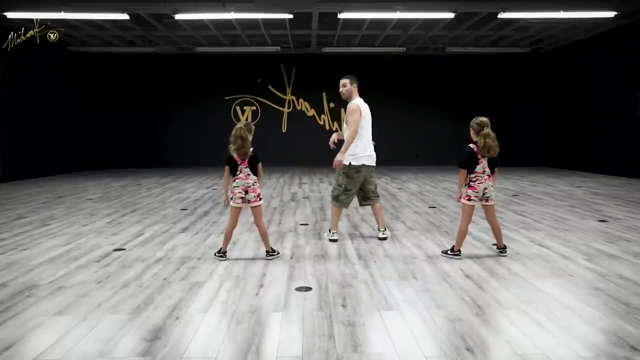 Okay, Drop the arms. The turn is going to be left leg, Right leg. we're facing the back. Good, Stay right there, Don't move. Once you're here, you're going to turn back around with the left leg. You want to put the feet together? 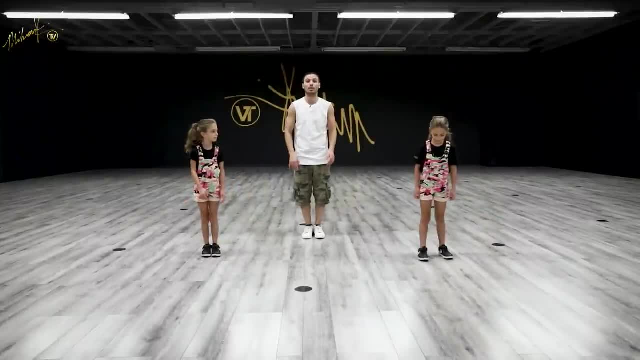 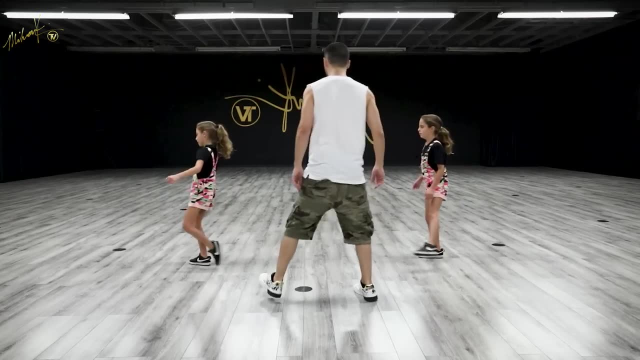 Whoop Feet together, Sophia Good. And then a quick jump out Out in Good One more time. Here we go, Step, We're going to go step, turning back together. Whoop Out in Good Again. 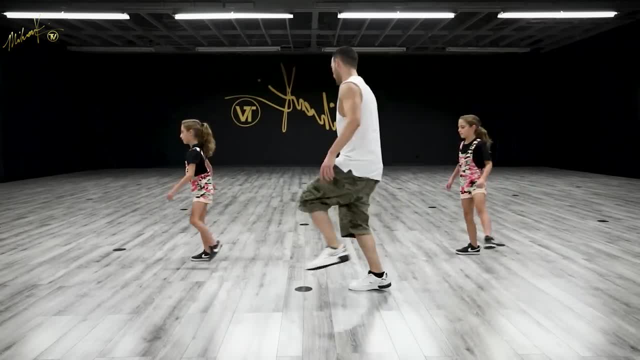 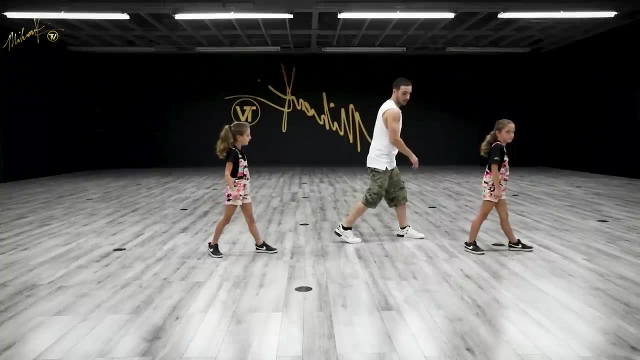 Six, seven, eight Go step and a step and together out in Good One more time. girls, Here we go: Five, six, seven, eight Go step, step together out in Good One more. 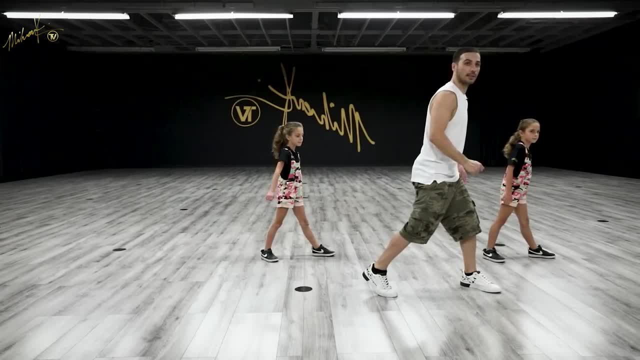 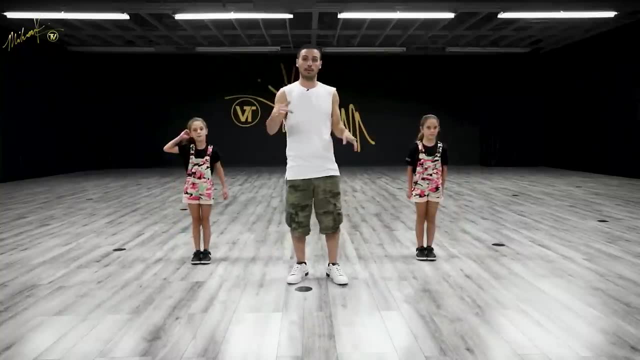 time. Here we go, and then we'll put it to the. we'll put it with the arms: okay, Six, seven, eight, Go, step, step, step out in. Alright, so now the arms. okay, We're going to punch with. 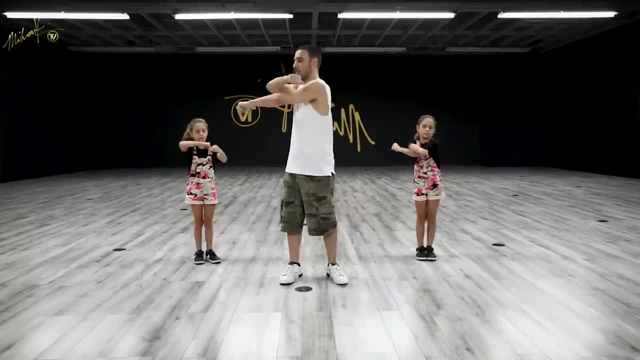 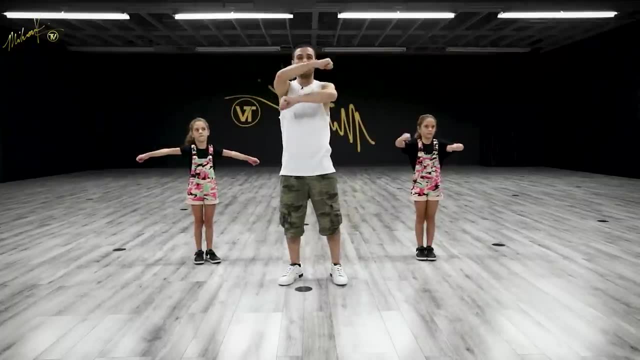 the right arm, It goes underneath the left arm. Let's do this a couple of times. Give me a little punch Punch. Good, So once we punch, we circle around, we open, and then the left arm is going to be on top, and then that. 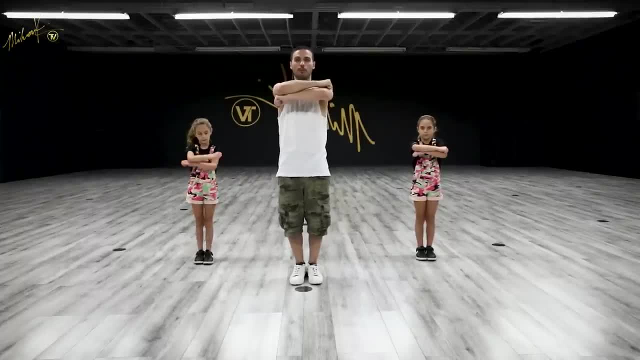 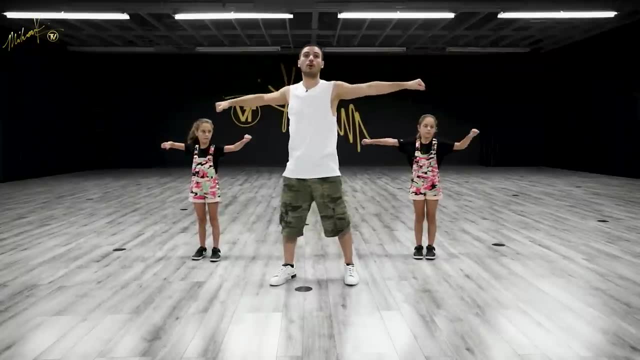 jump is going to be out in with the arms. So we finished here, if you remember, and then we're going to go boom, boom, Okay, So again, just arms. Right arm punches through, goes around, opens up Left. 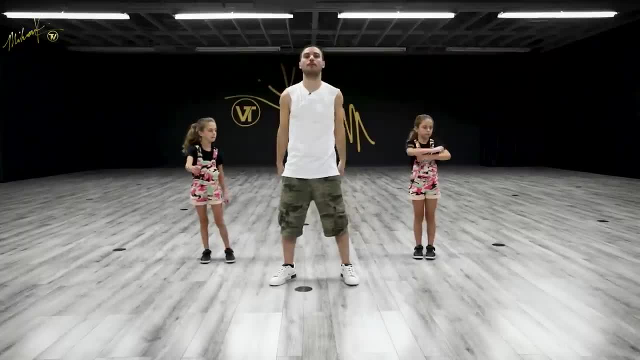 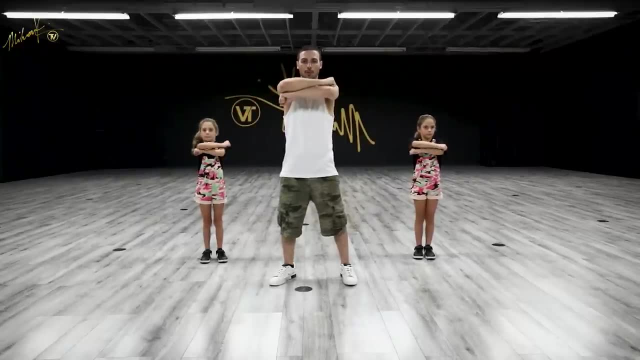 arm is on top. Out in Again. Five, six, seven, eight, Go punch around, boom, boom, boom Again Seven, eight. This is five, six, seven and eight. Okay, let's do it super slow. 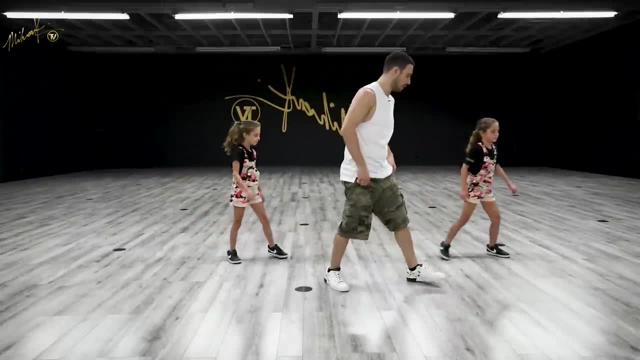 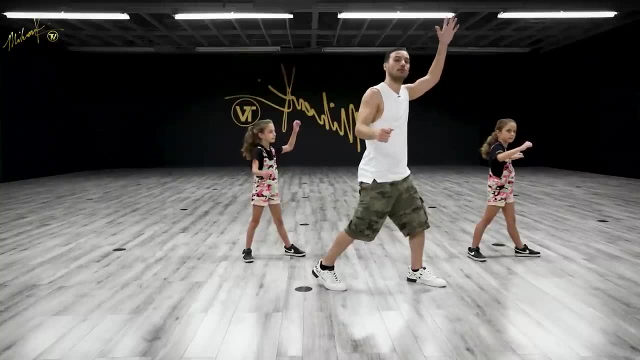 with the legs. It's going to be a little tricky. okay, Scoot over just a little bit. We finished right here. Everyone's arms are up. Good, Now on the step with the left leg, you're going to punch the right arm, We're going to do it. 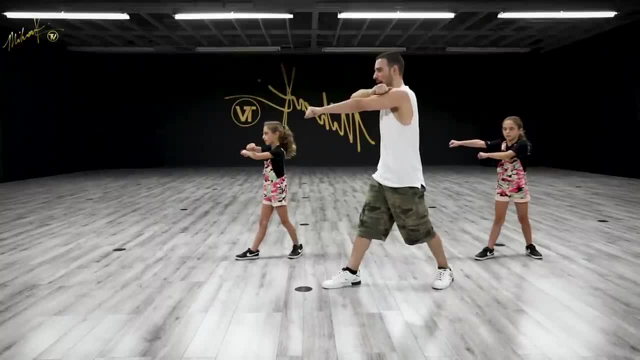 super slow. Seven, eight, This is five. Let's all hold that. Right arm is straight, Left arm is here. Now, as I circle around, I'm going to face the back. Both of my arms are going to be open. 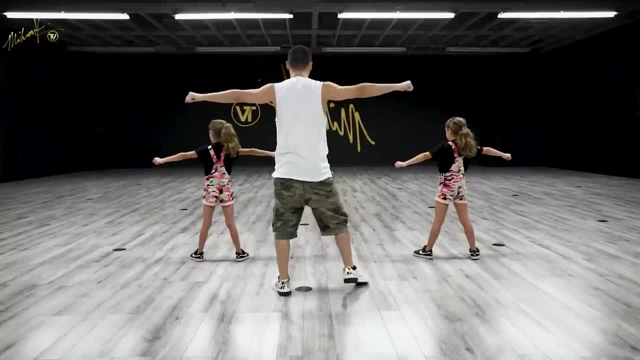 Boom, That's six. Now, when I turn around, right, I'm going to stay right here. Watch, watch, watch. Arms are up. As I turn to the left side, I'm going to bring the left leg, I'm going to put it together and my 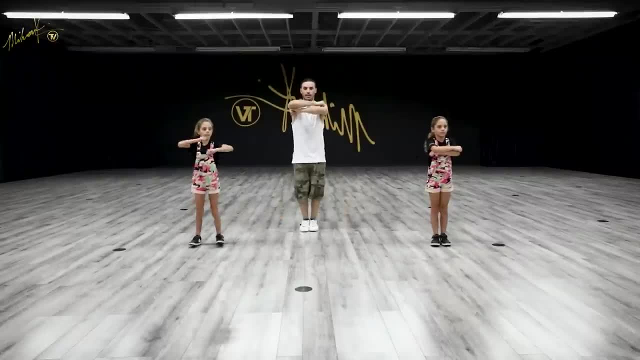 arms come together. Good, And then we're going to jump out and in. Good, One more time, Let's face the back. Just do the last part. So this is count six. We circle on seven and eight. Good, Now let's connect. 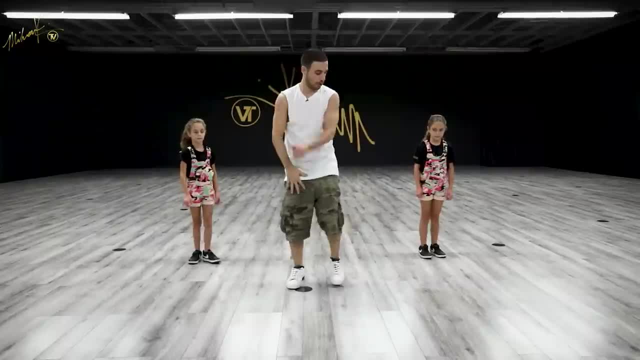 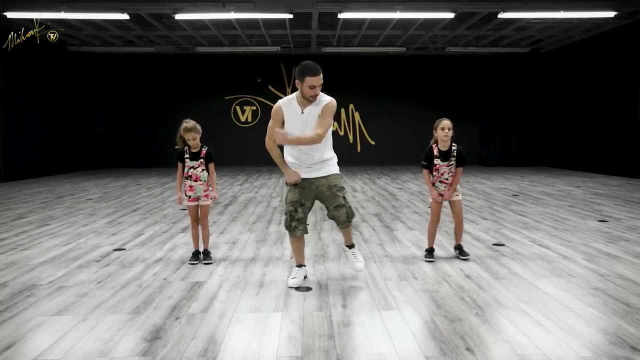 it together super slow moving back this way. Okay, We'll go five, six, seven, eight and start on one. Here we go Really slow: Five, six, seven, eight. This is five and six, seven and eight. 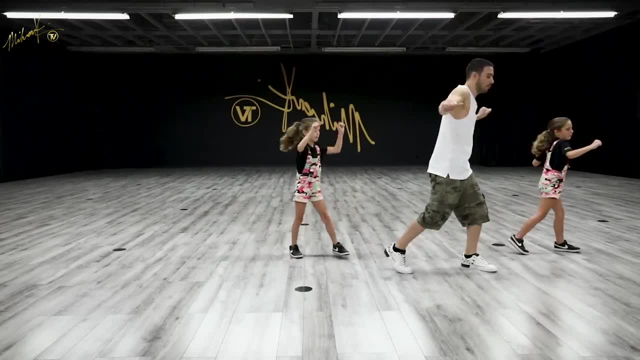 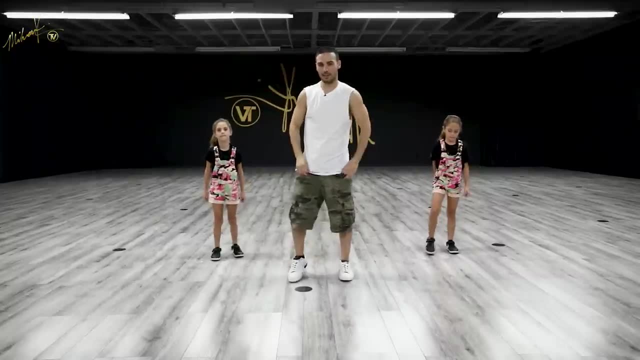 Step one, Step two, Step three, Turn four, Step five, six, seven, Boom, boom, Good, One more time. Here we go A couple of times- Let's work on that- from five, three, four, five. 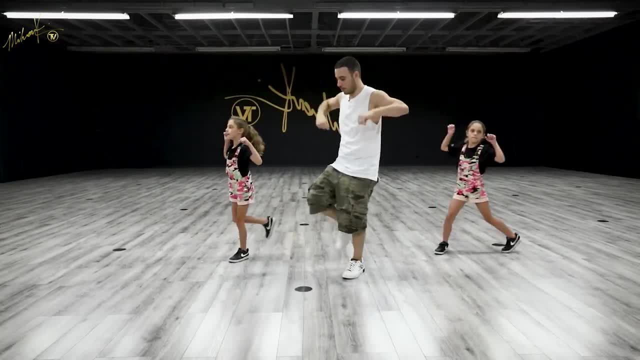 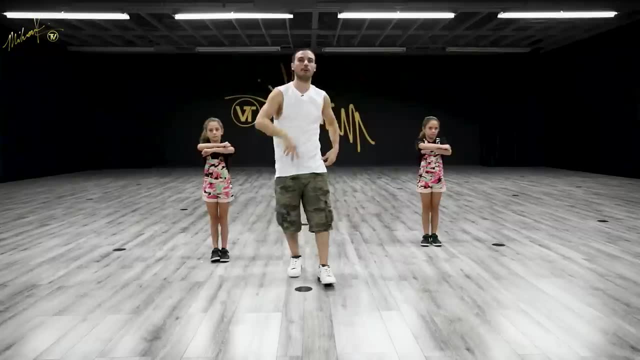 and a six, seven and a eight. Go one, Go two, Go three. Open four, Five, six, seven, Boom, boom Good. Two more times like that. Let's try to see if we could go a little faster. 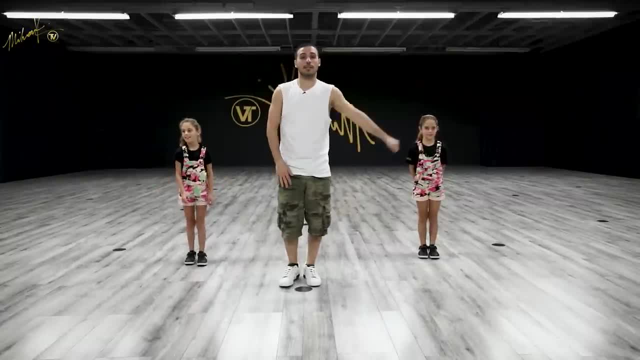 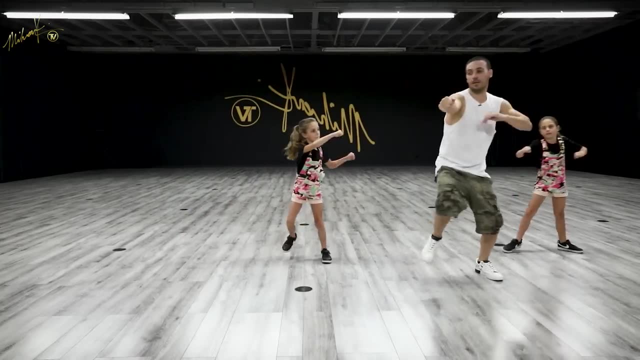 Faster, Here we go. Five, six, seven, eight Go five and a six, seven and a eight. Step one, Step two, Step three. Open four, Five, six, seven, Boom, boom, Nice, One more time, Here we go. 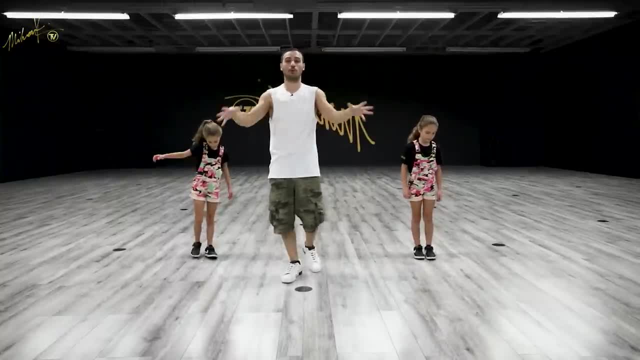 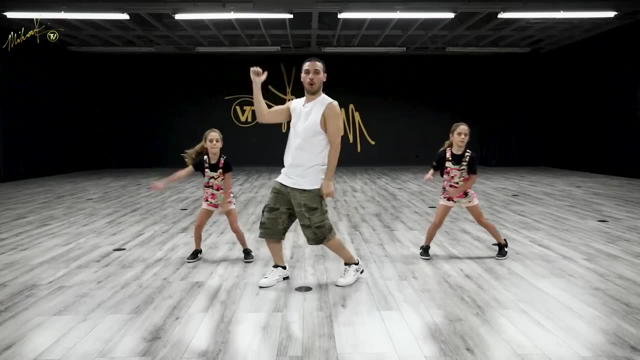 We're getting closer to music. Let's do this one more time, Take it back, Do a review of the whole routine. Five, six, seven, eight, Go, Hit Boom, Hit Go. one, two, three, four, five, six. 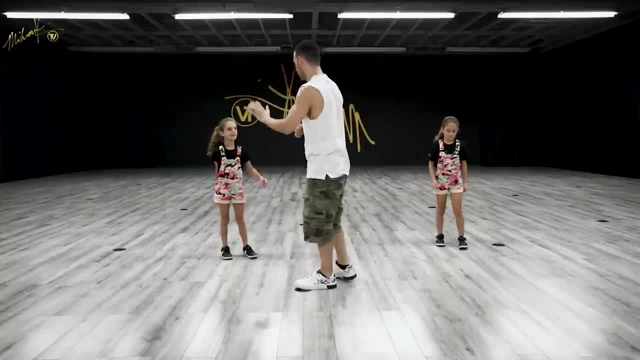 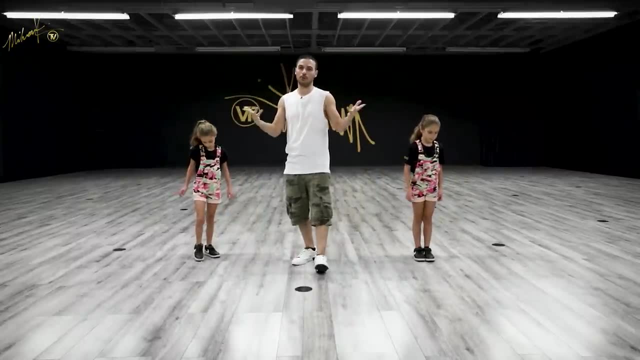 seven, Boom, boom, Nice. How do you feel, ladies? Good, Good, Let's go from the very top, Walk the whole thing slow, Walk it to tempo, Dance it with music. Here we go, Slow, walk Feet apart. 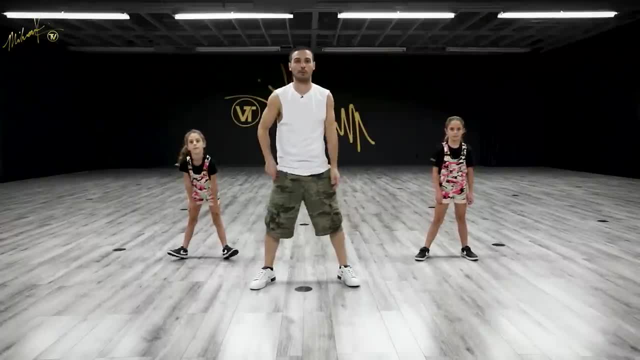 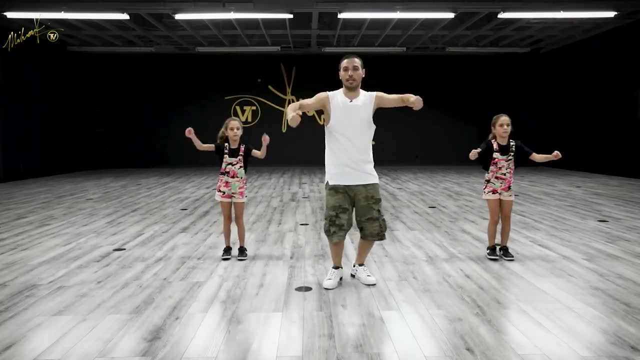 This is a quick review for you, for me, for the girls. everyone together, Six seven, eight. We're going bounce. Two, three, four, five, six, seven, eight. Step one: two, three, four, five. 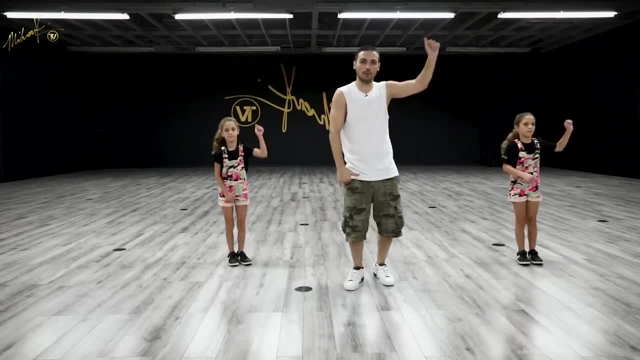 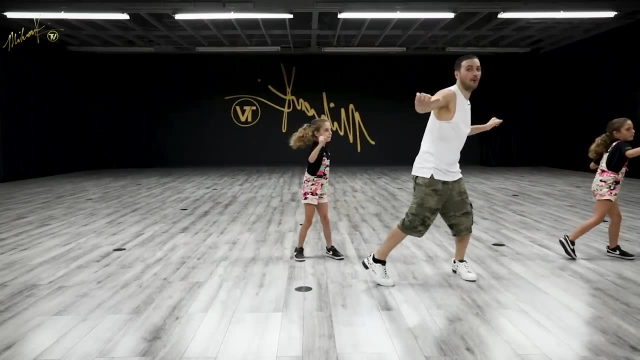 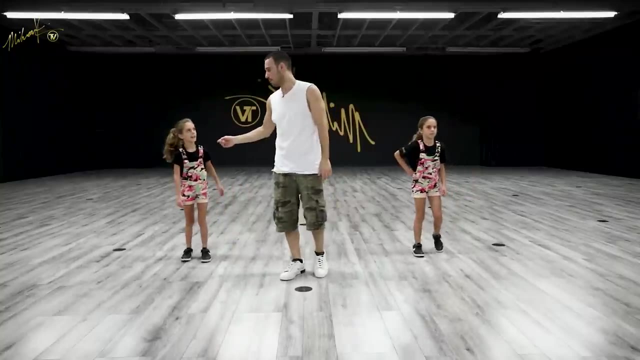 six, seven, eight Step: one, two, three, four, five, six and seven. Go. one, two, three, four, five, six, seven, Boom, boom, Nice, Let's see if we can speed that up Faster.